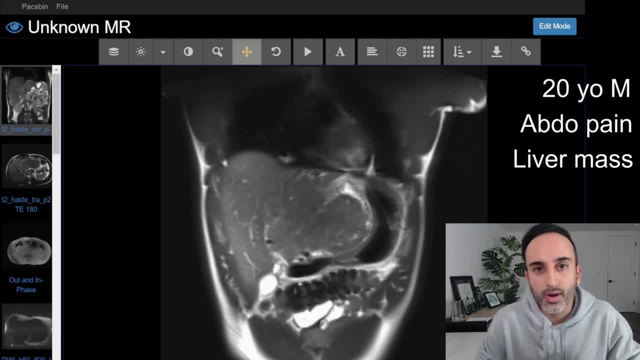 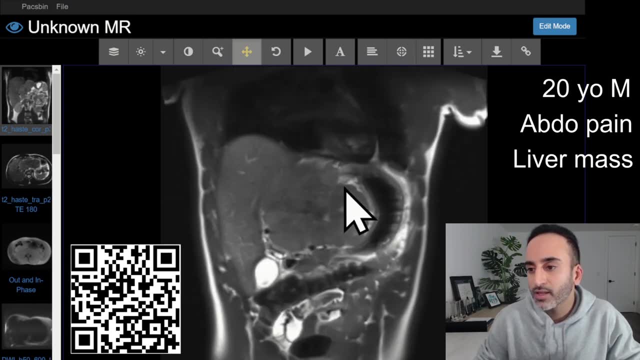 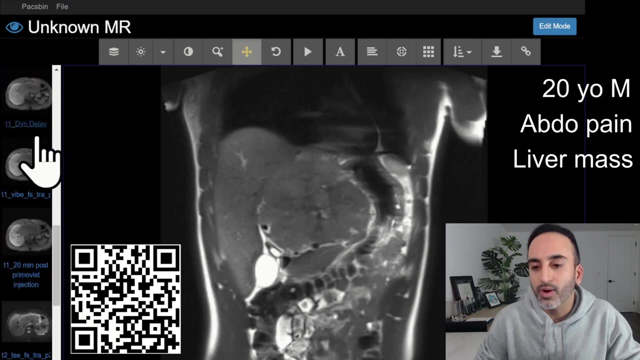 given the patient's age. but they suggest getting a liver MRI because it's big, to make sure that it's benign. And so this is the liver MRI in this patient and you can see that there's this big mass in the left lobe of the liver here, and all of the sequences as part of this MRI are here on. 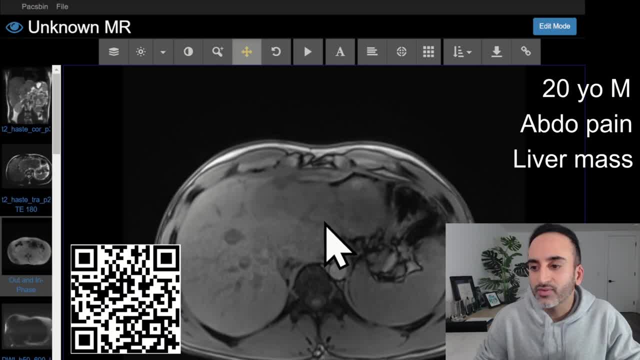 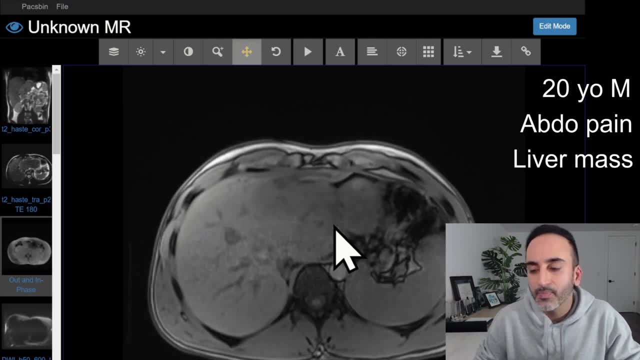 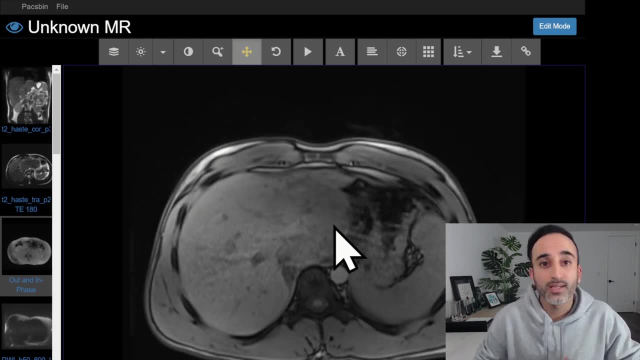 the right, And the appearance of this mass on each of these sequences is going to be a piece of the puzzle that helps us figure out what this mass actually is and what we think this mass is, and what we say about the mass is going to determine what happens next. So does this patient need to? 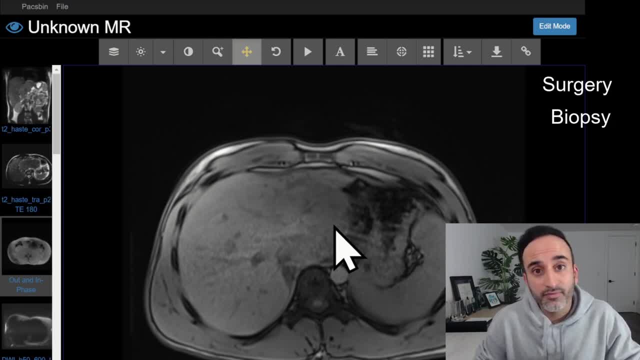 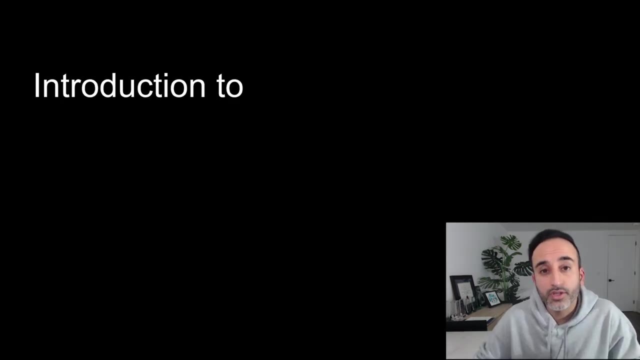 go to surgery. Do they need a biopsy of the lesion to figure out what it is? Is this benign and requires no further follow-up, or should we be following it up with imaging? So we're going to go through this case in further detail at the end of this video, This introductory. 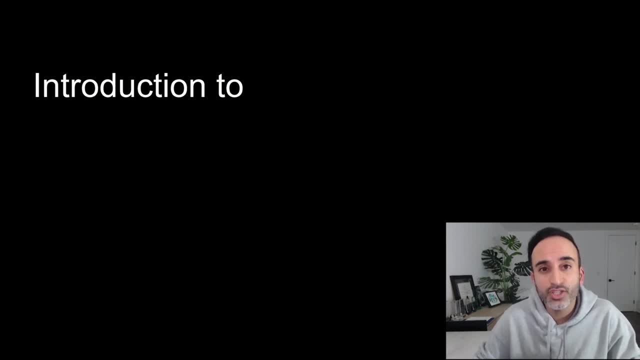 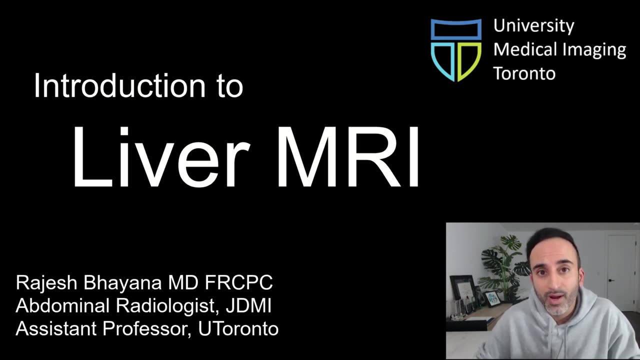 video is part of an interactive course that's designed to teach you how to read MRI of the liver. So by interactive, I mean that you'll be able to scroll through full MRI cases that are representative of the most important pathologies that you need to see, and we'll teach you how to. 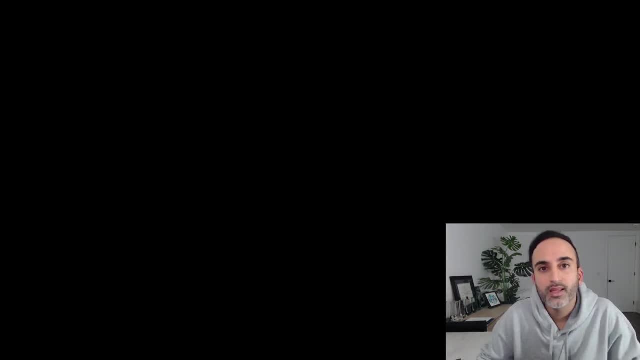 read MRI and we'll teach you everything that you need to know about each of these pathologies. The course is split into two parts, So this is the first part, which is an introductory video designed to teach you the basics, specifically what the sequences are in a typical routine liver MRI. 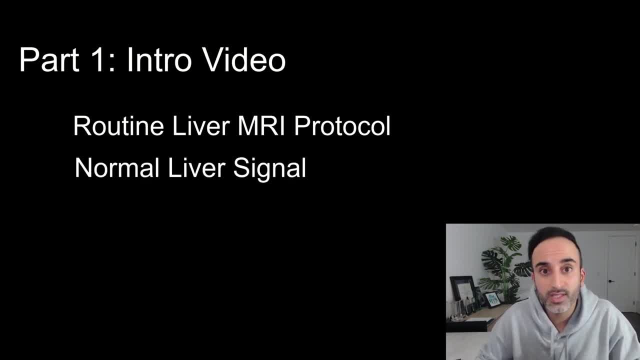 We also want to show you what the normal background liver looks like on all of the different sequences and what lesions look like in comparison, aka what you're looking for, And then we'll show you my approach to liver MRI. So basically going through what I use each sequence for when I'm looking at these studies. 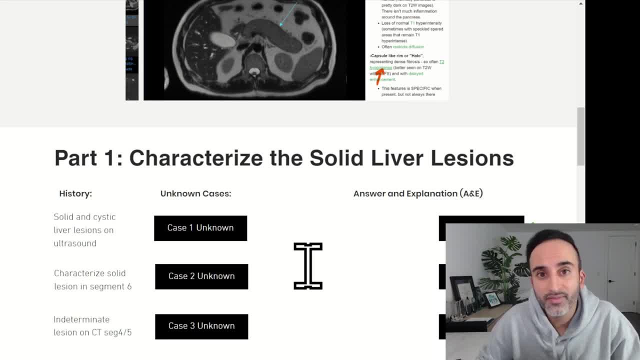 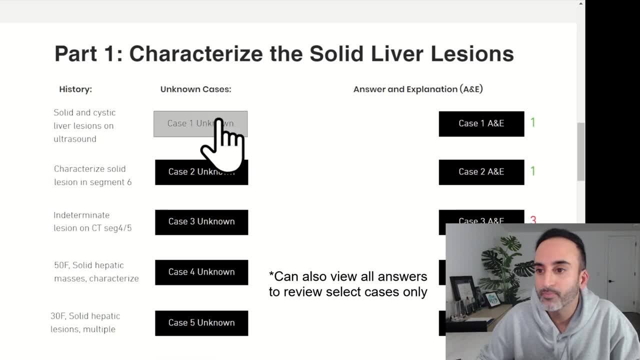 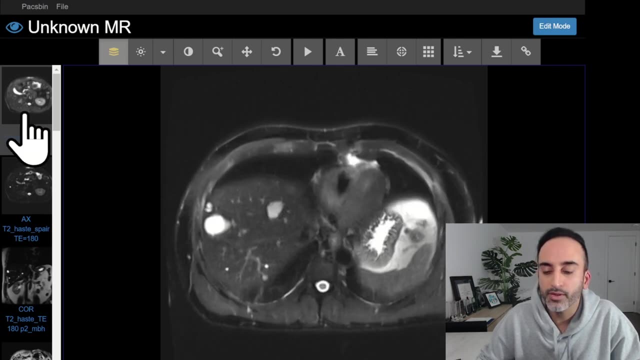 Then the second part is a series of over 25 carefully selected cases that you can scroll through and take a look at as unknowns. So, for example, here we have case one and if we click on the case we have the MRI images pop up with all of the sequences here on the left, and all of these. 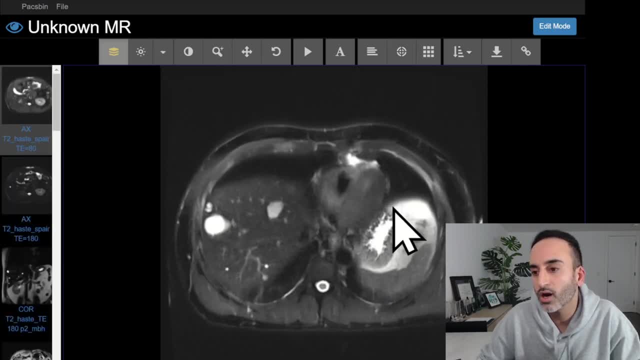 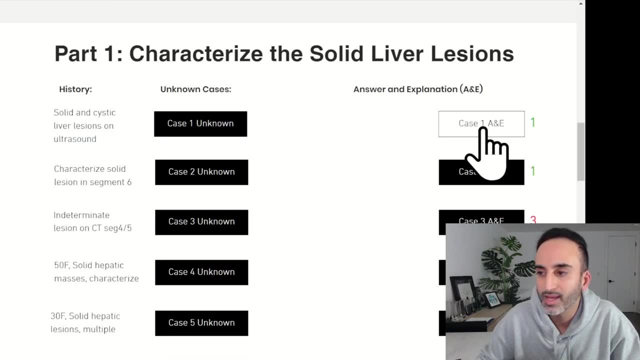 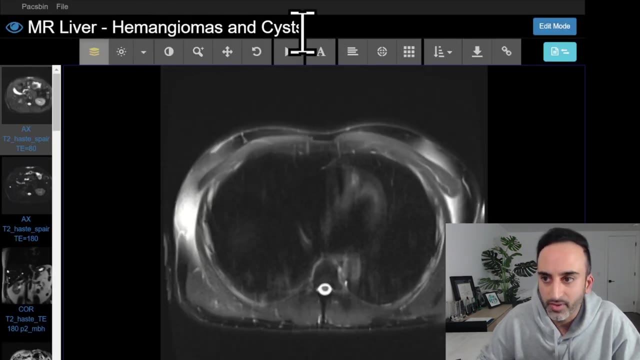 standard PACS tools across the top And you'll notice that there are several lesions here in the liver that require characterization. Each of the cases comes with answers and explanations. So, for example, if we click that here, we see that these are a bunch of. 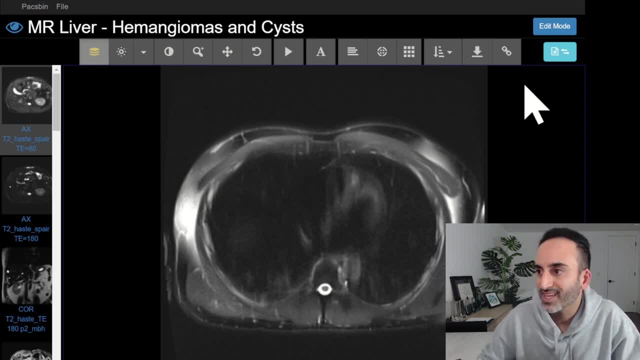 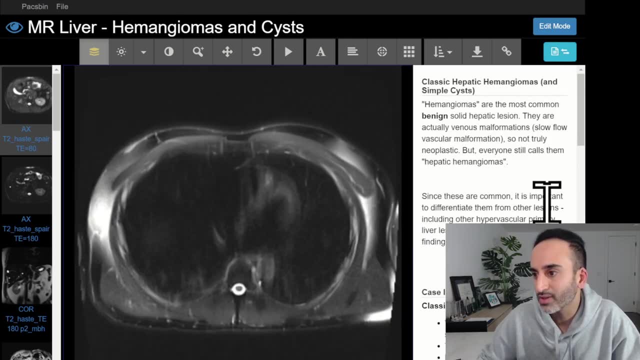 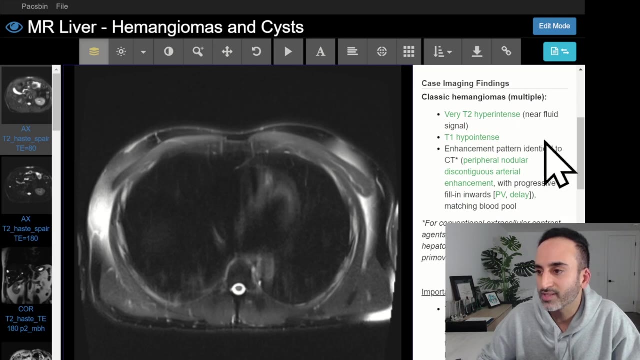 hemangiomas and cysts, so a very introductory and basic case. Then if we click on this blue square here in the top right, we have an explanation including everything you need to know about the particular pathology. So, for example, the imaging findings of a classic hemangioma here are outlined, and if you click on 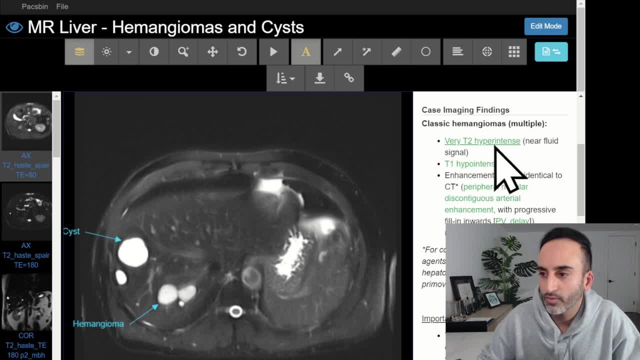 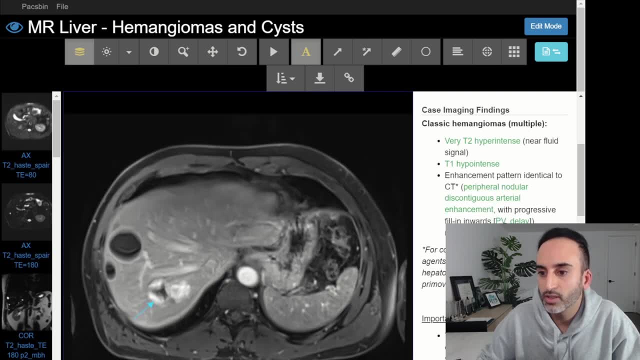 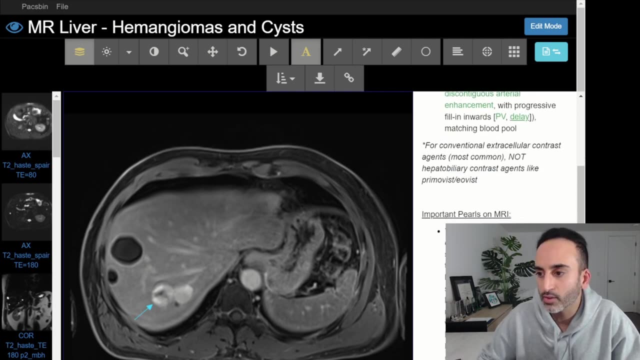 the links it'll take you to those imaging findings. So of course, classic hemangiomas are very T2 hyper intense and we go through the enhancement pattern here. on arterial, portal, venous and delayed phase imaging, We also go through some important pearls on MRI, including some more advanced MRI. 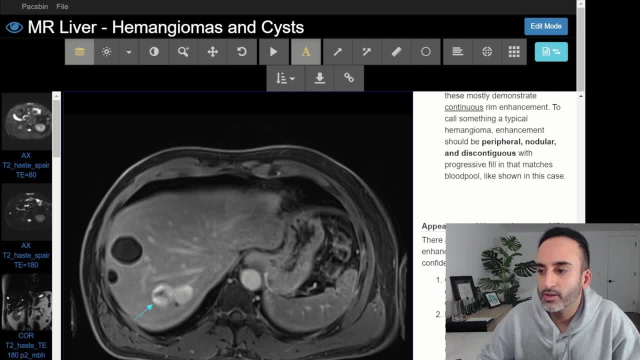 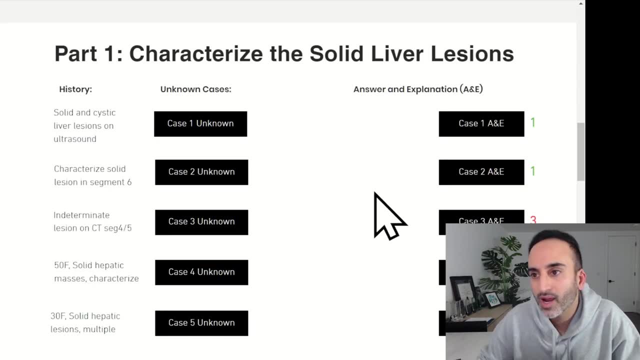 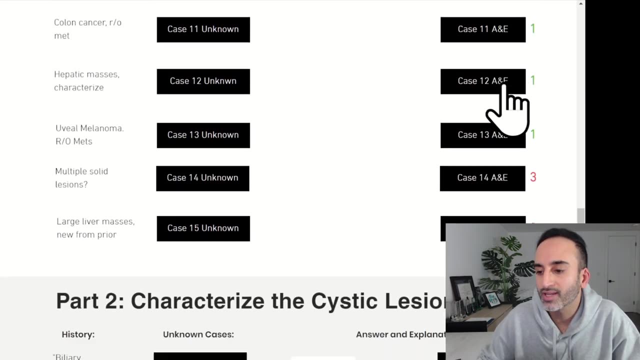 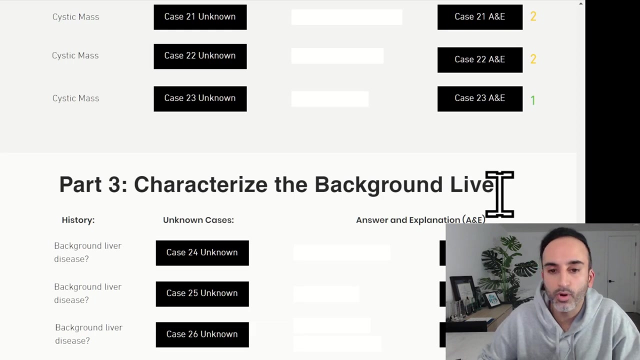 concepts, as well as the appearance of both typical and atypical hemangiomas on MRI. So for liver MRI, the cases focus on a few key areas, specifically characterizing solid liver lesions, characterizing cystic liver lesions and the characterization of the background liver, aka looking for diffuse liver diseases. So 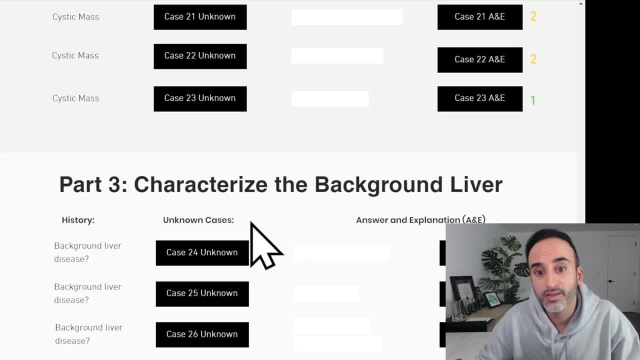 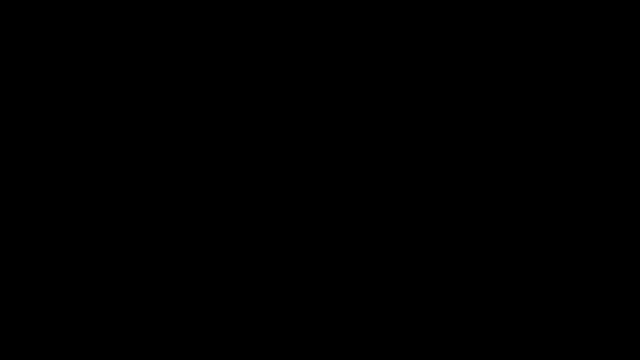 by the end of the course, you'll have seen all of the things that you need to see on liver MRI and to know to be able to interpret liver MRI efficiently and effectively. So this course includes all of the pathologies currently on the screen, and more, and can be accessed on our website. 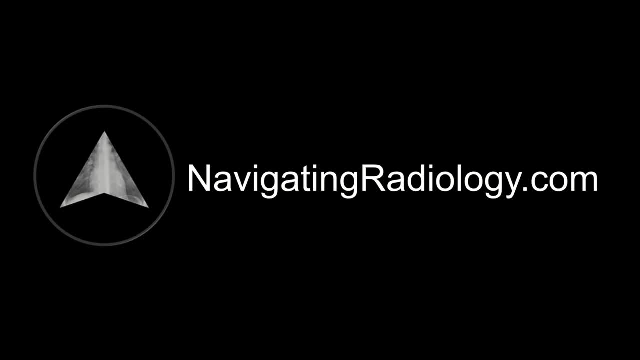 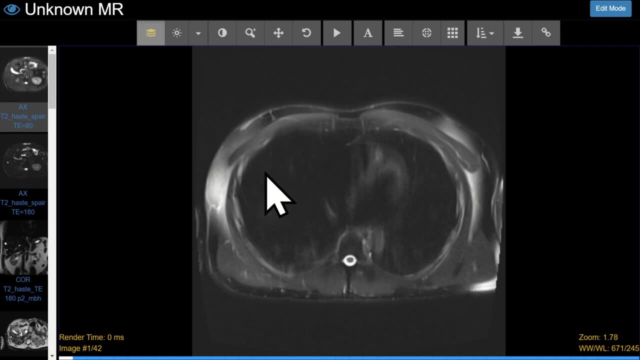 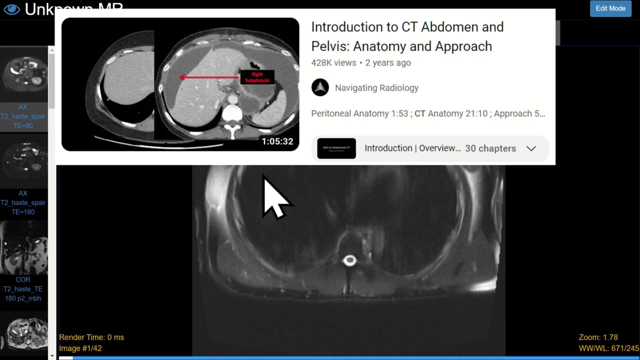 navigatingradiologycom, along with our other CT and MRI courses. Okay, so before taking this course, you should already know some MRI basics and anatomy. We cover basic liver anatomy in our CT abdomen and pelvis video, including liver, segmental and vascular anatomy. If liver MRI is new to you, I suggest starting out with our introduction to body MRI video. 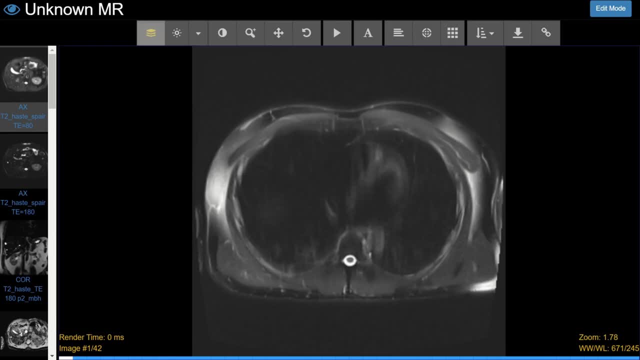 Okay, so let's start with the basics so we can get you working through the liver MRI cases as soon as possible. So let's open up that first case again. So, to follow along and scroll through this case, you can use the QR code on the screen to open up the case on your phone or use the link in the. 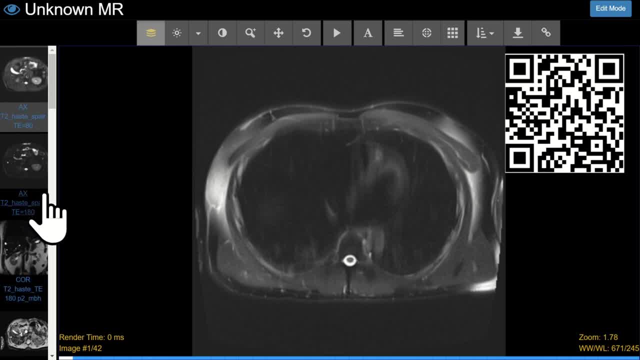 description. So on the left here we have all of the MRI sequences that are part of this routine liver MRI protocol. So scrolling through and looking at all these sequences it can be a little bit overwhelming at first, but if we break it down it's really not that bad. There are four groups that we can put each of. 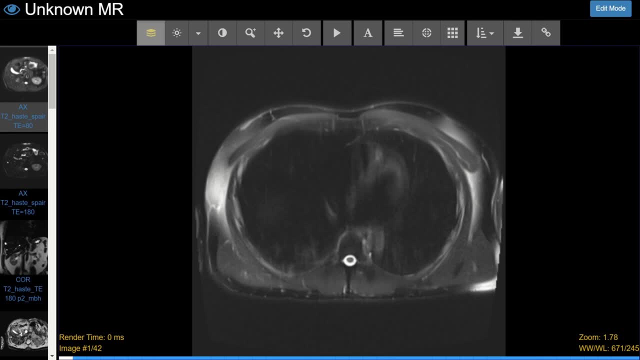 these sequences in and as we go through each sequence we'll pay special attention to the appearance of the normal liver and what we use each sequence for. So the first group of sequences that we're going to talk about are the T2 weighted sequences. So this is an axial T2 weighted sequence. 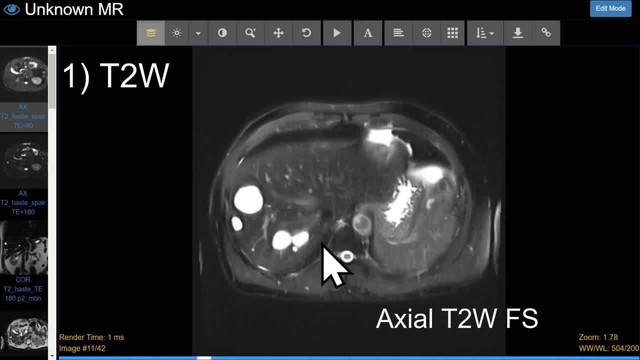 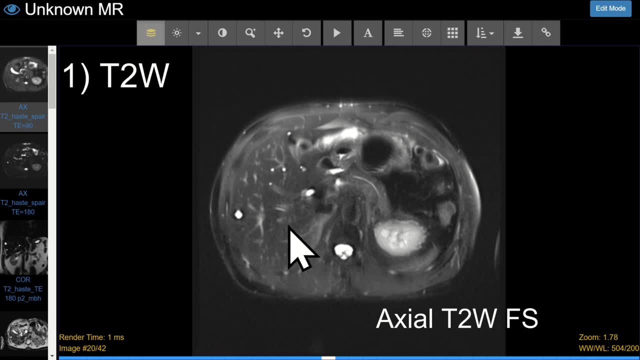 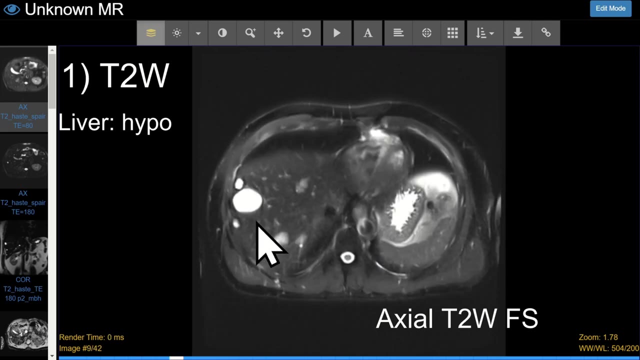 so notice that the subcutaneous fat is all very dark or hypo intense and notice fluid like the CSF here or the fluid in the gallbladder is very bright. Also, notice that the liver is relatively hypo intense on T2 weighted images, so it's pretty dark Most of the lesions that we see in the liver. 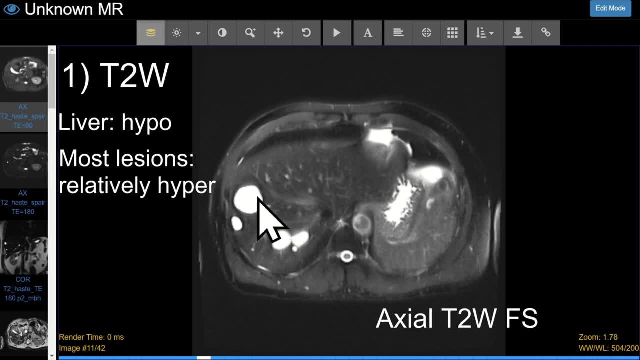 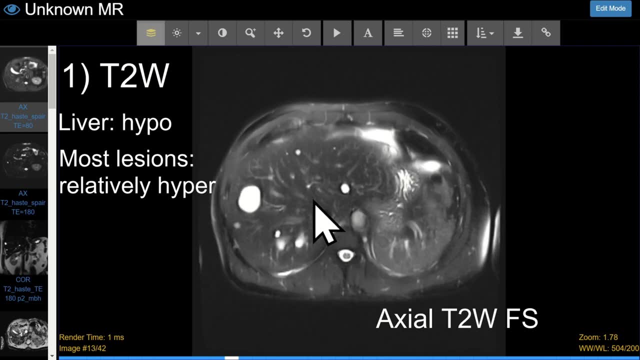 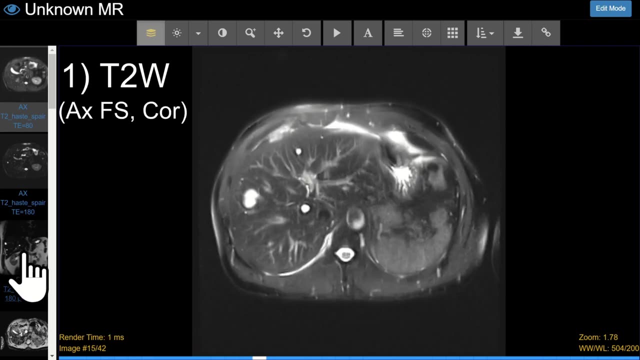 here, or in most cases, are going to be relatively hyper intense to background liver, ie they're often going to stand out as relatively bright on a dark background in most cases. So in a routine liver protocol we usually perform T2 weighted sequences in axial and coronal, with at least one of them with fat suppression and one of them without. so 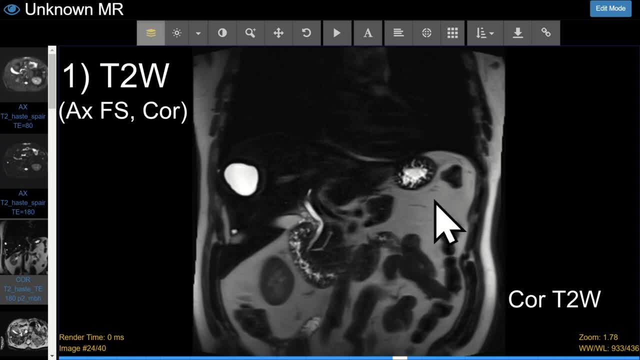 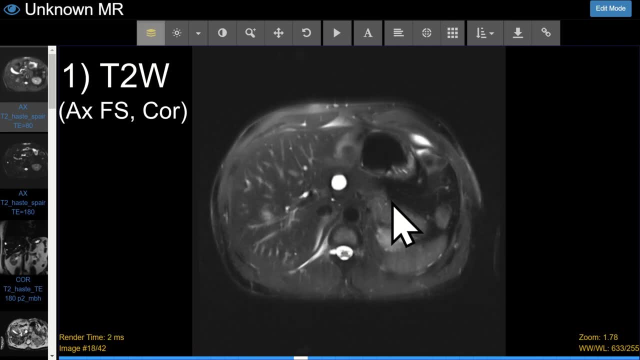 notice that this coronal sequence is performed without fat suppression, so the fat is still hyper intense. So sequences with fat suppression, like this axial, are going to be more sensitive to picking up fluid signal because fluid is relatively bright on a darker, blacker background. but we perform. 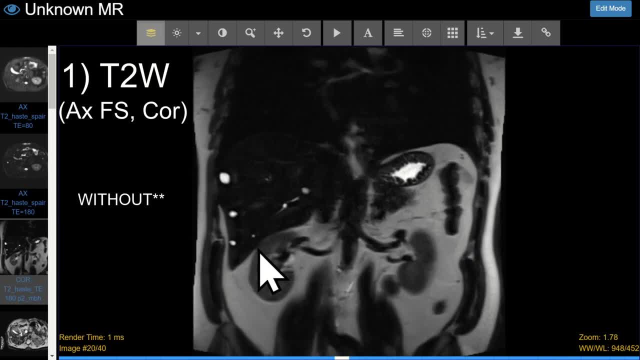 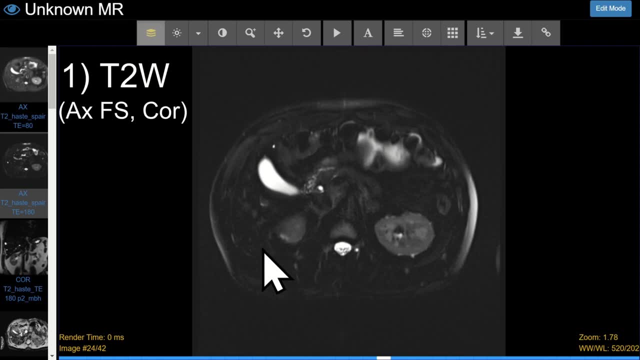 sequences with fat suppression to better define the anatomy. so, for example, you can see where the liver ends and where the fat starts here. and if I looked at this axial with fat suppression, it's harder to tell, for example, where the liver ends and where the fat starts. So, although we cover 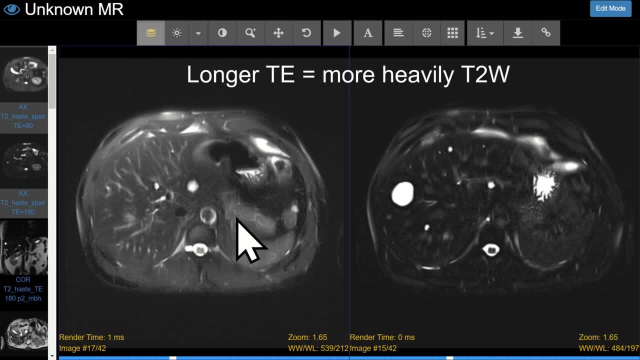 this in our intro to body MR video. remember that longer TEs are going to make the image more heavily T2 weighted. In other words, as TE gets longer or the echo time gets longer, fluid maintains its signal and the T2 is going to be more active and more active in the body and that's how we're going to see the t2 in the T2-weighted image. 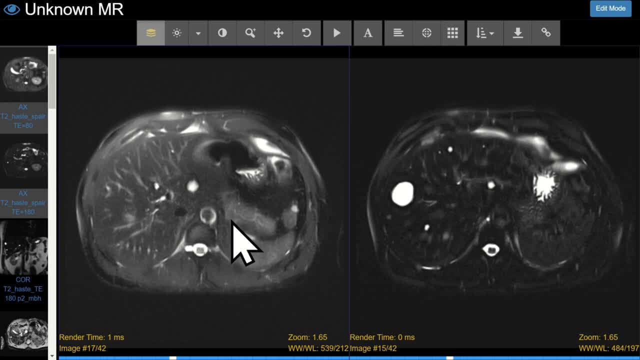 stays very bright and everything else gets darker. so, for example, if you look at these first two sequences in this particular protocol and we put them side by side, you'll notice that they're both t2 weighted sequences with fat suppression and they're both performed in the axial plane. 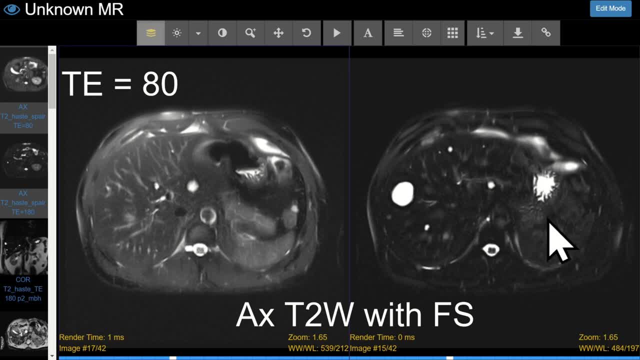 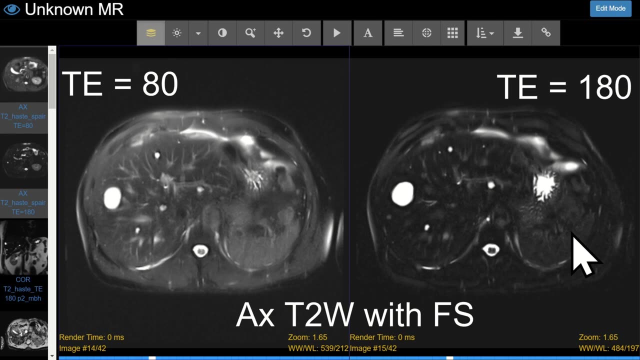 but the first here on the left has a te of 80 and the second here on the right has a te of 180 or it's longer. so notice that with a longer te the fluid maintains its signal here, but everything else gets darker or loses signal and, as i showed earlier, in this case, this anterior 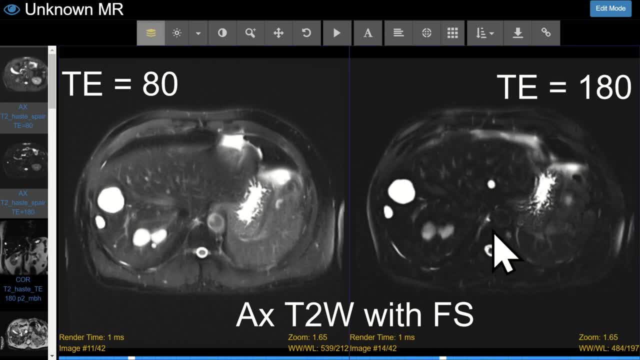 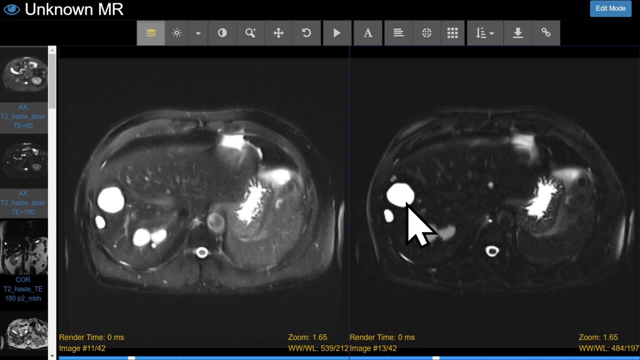 lesion here is a cyst and this posterior lesion here is a hemangioma. notice that on the shorter te they have more similar signal, but on the longer te the hemangioma has lost some signal relative to the very bright cyst. it's also worth noting- although we're going to discuss biliary imaging in another video- 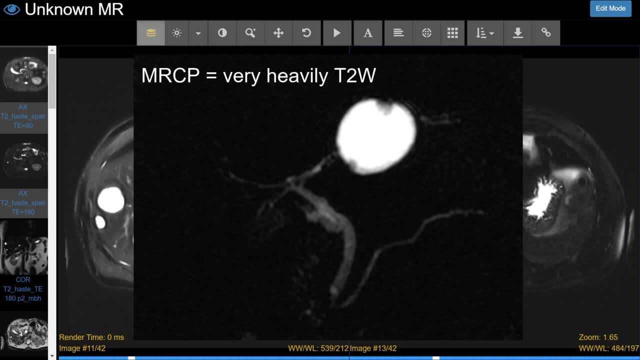 mrcp images are just very heavily t2-weighted images, ie they have a very long te, so you can see the anatomy of the fluid-filled structures very well, so for example, the biliary system, and depending on the protocol, you may also have mrcp images on our routine. 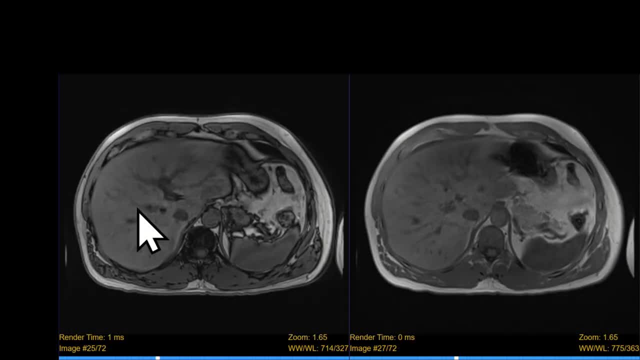 liver mri protocol. we do not, okay. so we've talked about the first group of sequences, the t2 weighted images. now let's move on to the t1 weighted images. so again, we covered these in more detail in the body mr intro video, but as a reminder, we performed 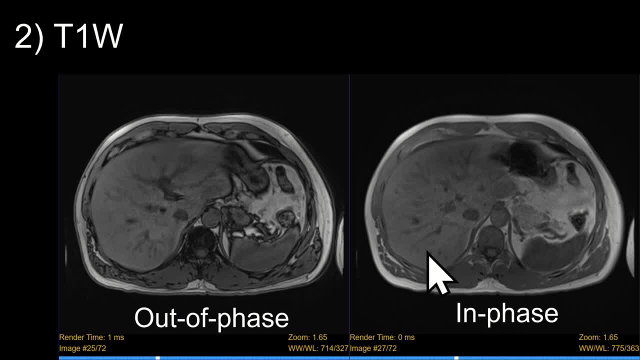 in and out of phase acquisitions. so here we have the t1 in phase on the right and then the out of phase here on the left, easily identified by this india ink artifact. so these images can be used to assess for intravoxel fat and susceptibility artifact from things. 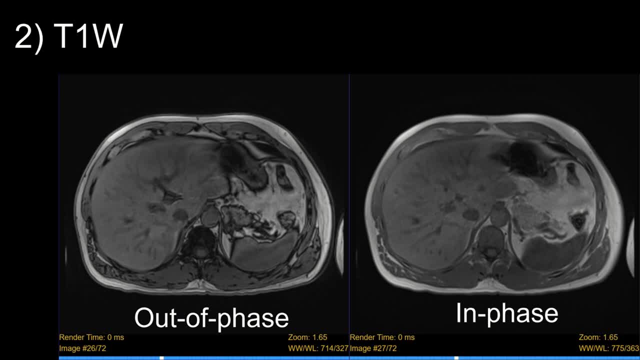 like iron, metal, air etc. so, for example, we can look for fatty liver or iron loading. so we want to point out those three areas that we study: bad liver器 fat, along with TMVWs orい in the background liver or fat content in lesions, for example. So fat in a focal liver, lesion of 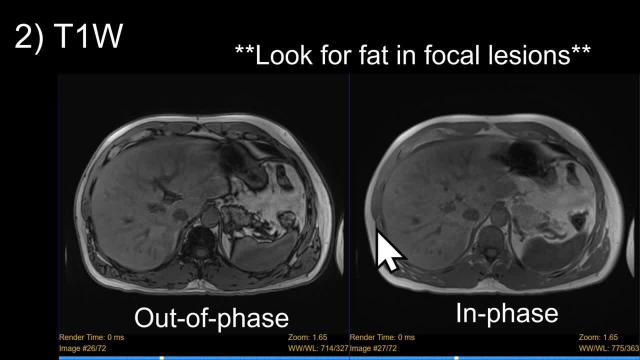 course is going to significantly change the differential for the lesion. so it's important to look for As a reminder: if we compare the in and out of phase images, voxels with both fat and water protons are going to decrease in signal on the out of phase images, hence the India ink. 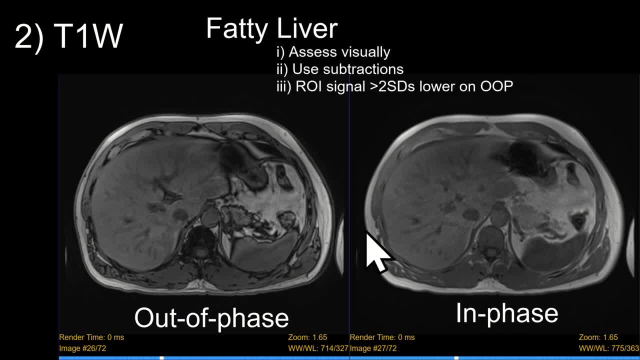 artifact at the margins of the organ. So for fatty liver, for example, the liver is going to be darker on the out of phase compared to the in phase sequence. Also, remember that the out of phase acquisition is performed first or before the in phase sequence. so when we have susceptibility, 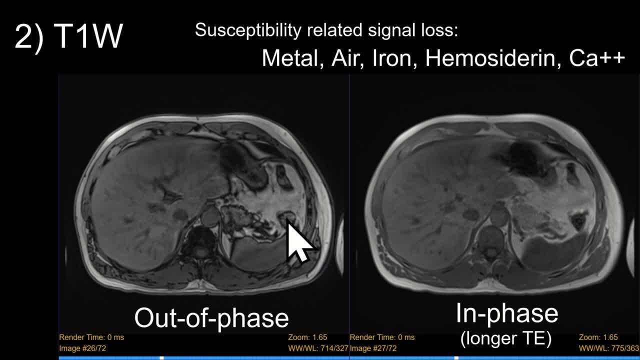 artifact from something like metal air. iron calcification susceptibility leads to a loss in signal at that site over time. so since in phase is acquired later, these areas will be darker and maybe even larger on the in phase sequence. So, for example, if there was iron loading in the liver, the liver would be darker on the in phase. 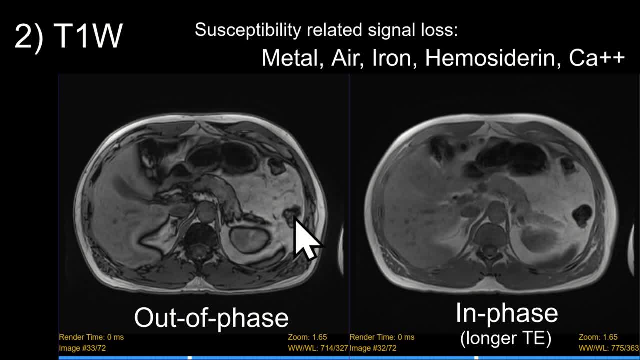 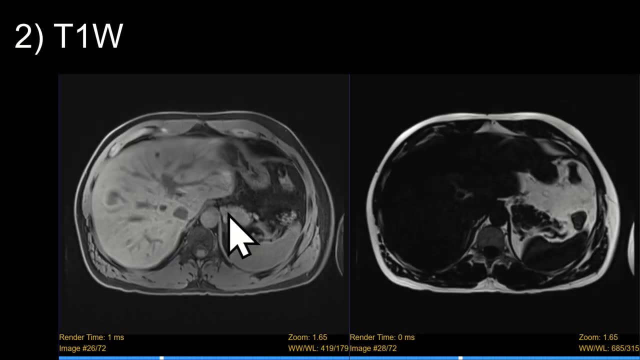 than the out of phase. So notice here, for example, on the out of phase, we have some gas here in the colon, as expected, and notice how it's darker and larger on the in phase image related to the susceptibility artifact. Okay, and next, from the in and out of phase acquisition using the Dixon. 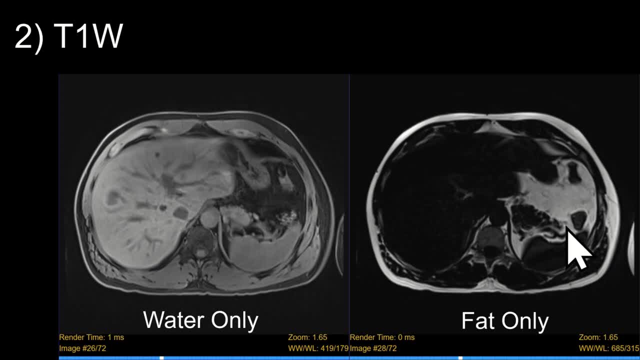 method we can calculate water only and fat only images. So, for example, if there was iron loading in the liver, we can calculate water only and fat only images. So the water only image is a nice T1 fat suppressed image. Notice that the fat is very nicely suppressed over here on this image. on the 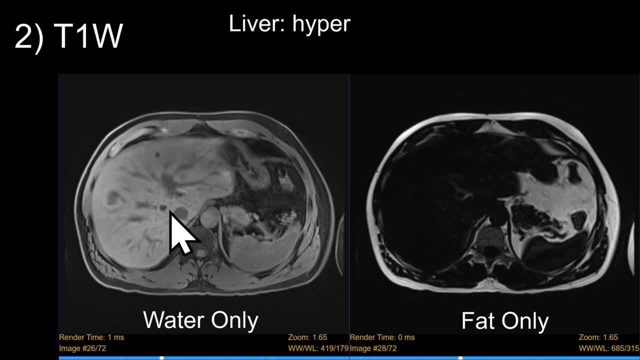 left. Also notice that the background liver here is actually pretty bright on these T1 weighted images. so most lesions are going to be relatively hypo intense to background liver. but also things that are very T1 hyper intense are going to stand out nicely on this T1 weighted fat suppressed. 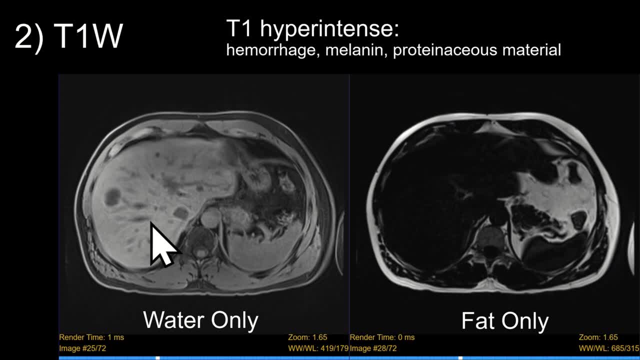 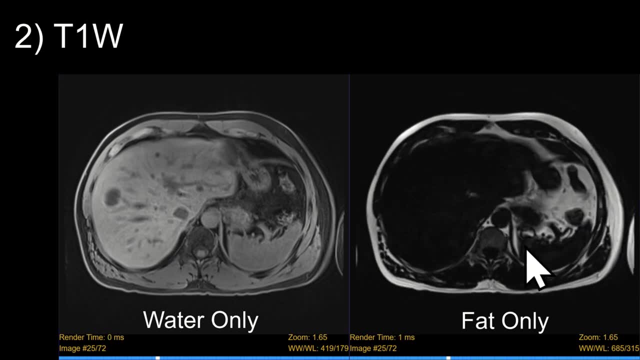 sequence. Remember the things that are T1 hyper intense are going to stand out nicely on this: T1 hyper intense, most importantly for liver MRI hemorrhage, melanin and other proteinaceous material. This image here on the right is the fat only image and, as a reminder, the fat only is going. 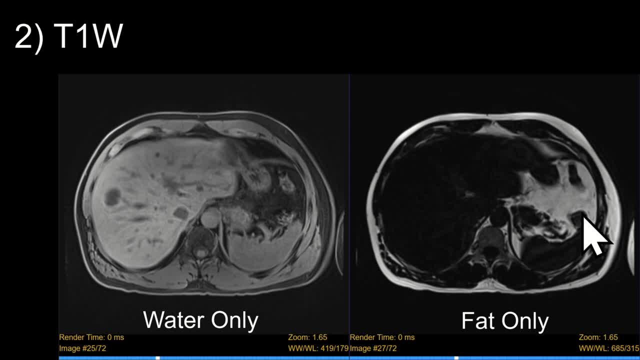 to show you both bulk fat and intravoxel fat. So this sequence is helpful to quickly identify fat in lesions and also to look at the bones. So normal fatty marrow is going to be relatively hyper intense. so marrow replacing lesions are going to show up as relatively hypo intense. 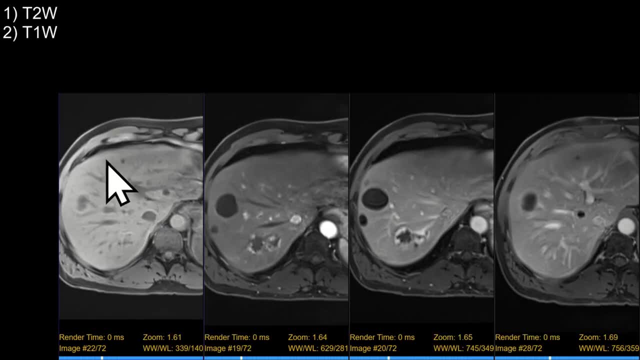 Okay, so so far we've talked about our T2 weighted sequences and our T1 weighted sequences, including the in and out of phase and downstream sequences. So third, and not an order of acquisition, but to logically remember all of the sequences that you need to account for is our T1 pre and. 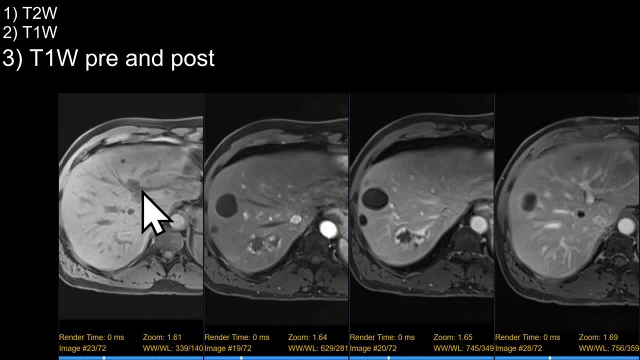 post contrast images, which again is logical. so we're going to give contrast or gadolinium, So we're going to have both pre and post gadolinium images here. So here on the left, we have our axial pre contrast image and then gadolinium is given and we have acquisitions. 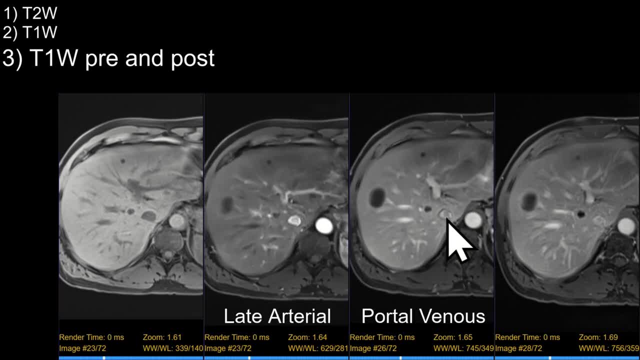 in the late arterial phase, portal venous phase and delayed phase. We also acquire a delay in the chronoplane that we'll look at in a bit. but notice that all of these are fat suppressed, of course, so an MRI signal intensity is relative. So if we want gadolinium, which is very T1 hyper intense, 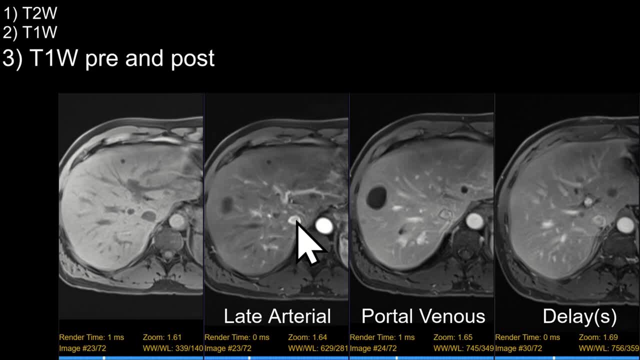 to stand out as the brightest thing on the image. then we want to suppress the very bright fat signal so that we can actually see what is enhancing. But let's talk a little bit more about these phases. So first, starting with the late arterial phase, notice that the 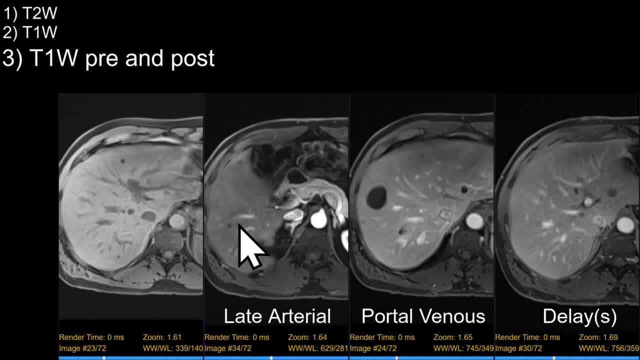 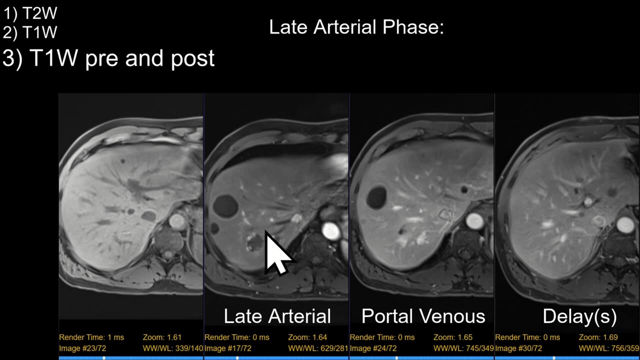 background, liver is still relatively hypo intense, so hyper vascular focal liver lesions are going to stand out as relatively bright on a darker background. Very importantly, the timing of this acquisition in late arterial phase is very important in liver imaging To detect HCC and other hyper vascular lesions. so poor timing of the later arterial phase. 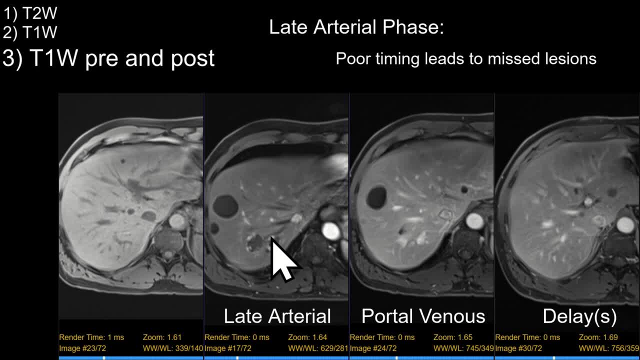 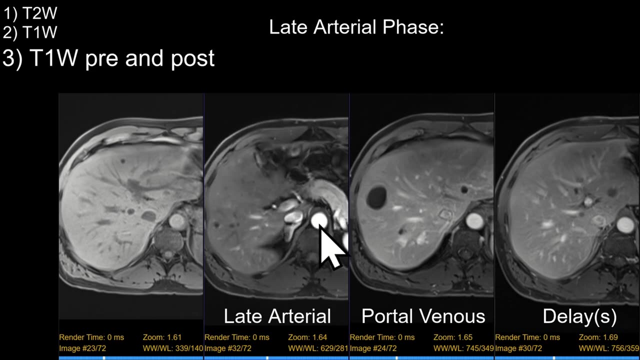 either too early or too late can and will lead to missing important lesions like HCC or hepatocellular carcinoma. So how do we know if it's well timed? So, in short, a good arterial phase should have, of course, opacification of the arteries and the portal vein, but not yet opacification of. 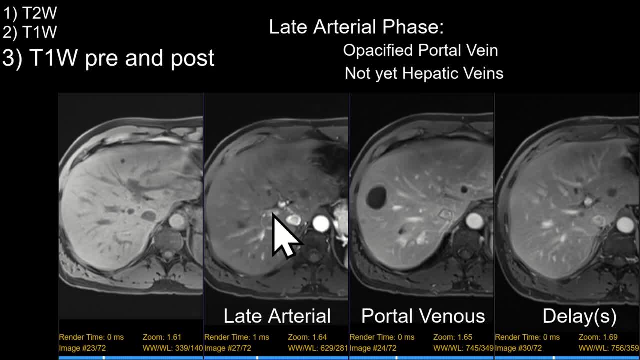 the hepatocellular vein. So if we want to know if it's well timed, then we need to have a good look at the epatic veins. If the portal vein is not yet opacified at all, then it's too early, and if the hepatic veins are already opacified, then it's too late. So this is a key concept that you need. 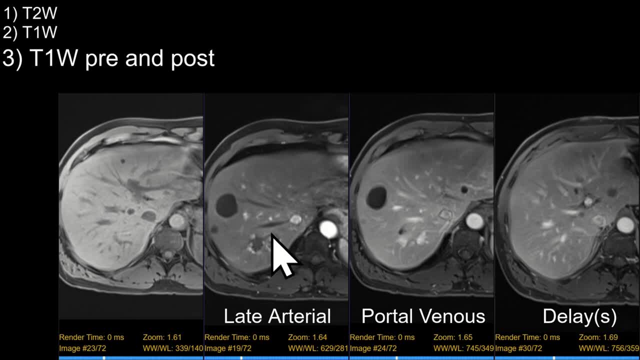 to remember when it comes to liver imaging and for this reason, HCC specific MRI liver protocols will often acquire more than one arterial phase back to back to increase the chance that we have a well-timed late arterial phase acquisition and have the best chance of detecting the 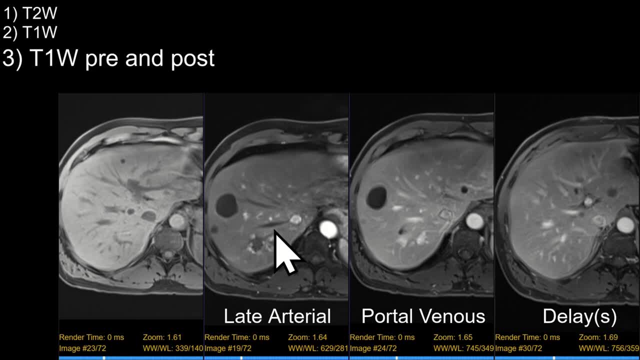 hypervascular lesions like HCC. This third image here is the portal venous acquisition. Notice that the portal vein is opacified, but the hepatic veins are also opacified. Also, notice that the background liver is now brighter, so hypovascular lesions are going to stand out very well on the 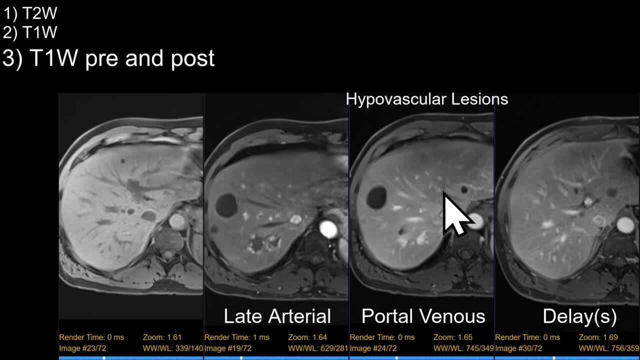 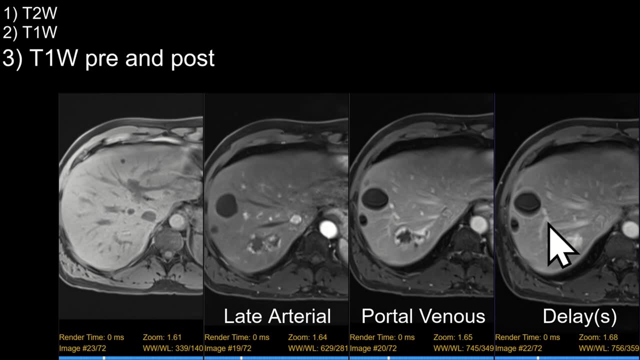 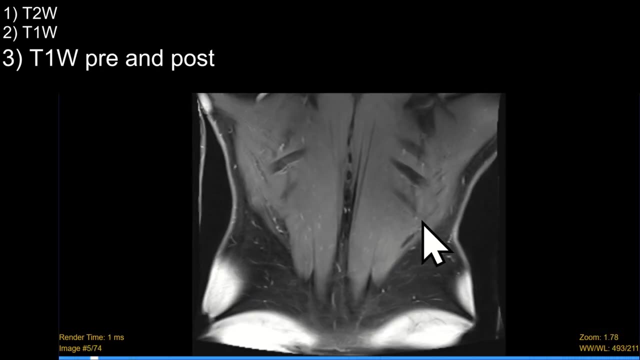 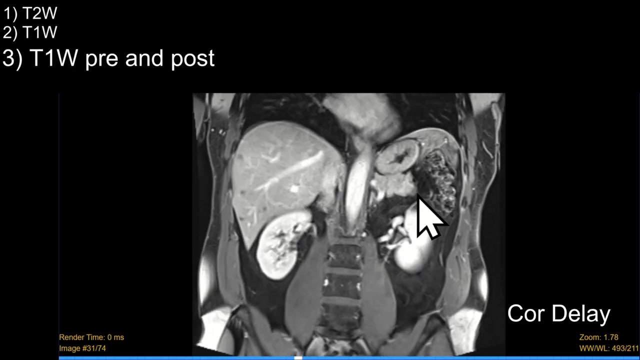 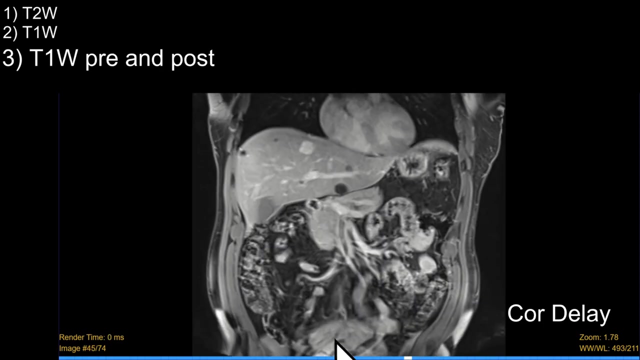 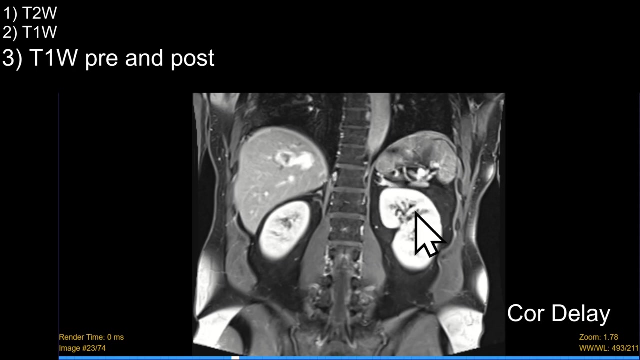 portal venous phase as relatively dark on a brighter background, Of course, the enhancement pattern of lesions over time from arterial to portal venous to delay is very important. So if the portal venous phase is very important in accurately characterizing liver lesions- just like on CT, also very important- the delayed coronal acquisition often covers more anatomy than the axial sequences. so it's a great sequence to catch incidental findings in the lungs, in the breasts, in the pelvis or partially imaged pelvis and in the bones. So you need to look for these things on every case. on this coronal post-gad image. 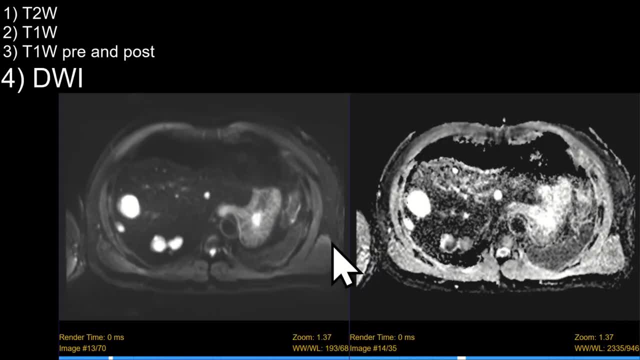 Okay, and lastly, fourth, we have our diffusion weighted images, which again we covered in greater detail in our introduction to body MRI video. but this includes the DWI acquisitions with multiple B values. so here is a lower B value acquisition, aka there's less diffusion weighting, It almost 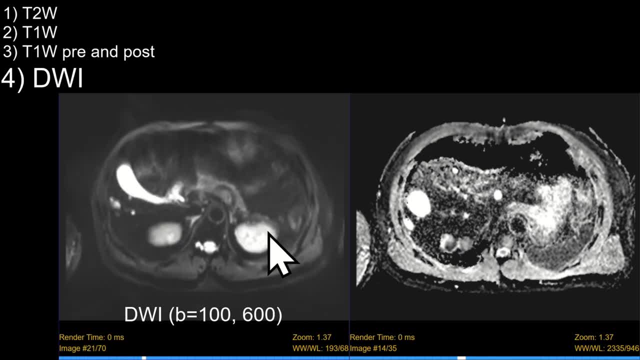 looks like a T2 fat sat or a poor man's T2.. Notice that the simple fluid is going to be very bright here. If we keep scrolling, we get the higher B value acquisition, which is more diffusion weighted, And then from that we can calculate the ADC. This is what it looks like here on the right. 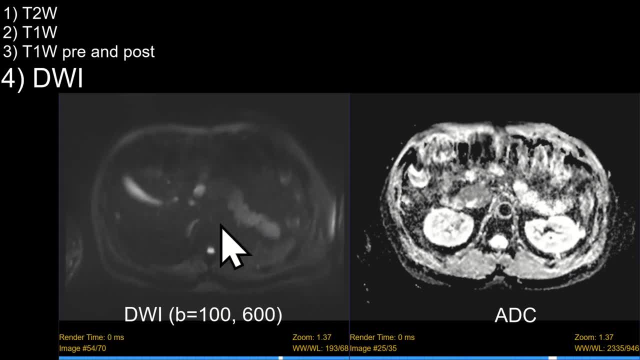 And so things that restrict diffusion should be bright on higher B value DWI images and darker on ADC. And again, this is covered in greater detail in the body MRI video. So many solid malignancies are going to restrict diffusion. Okay, so with all of these sequences, we've covered. 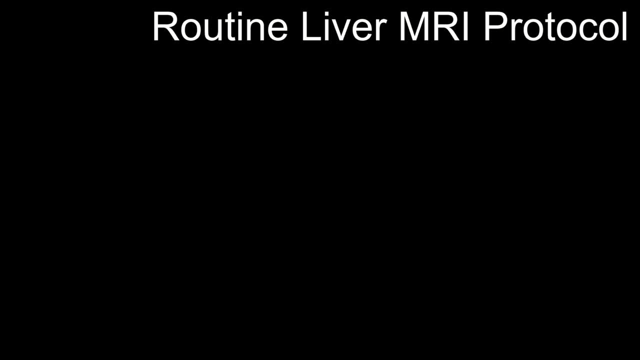 quite a bit, but the protocol isn't really as complex as it may seem at first. So again, a typical liver MRI routine protocol includes T2 weighted sequences in the axial and coronal plane plus minus more heavily T2 weighted sequences with very long TEs. like MRCP, We have our T1 weighted sequences including the in and 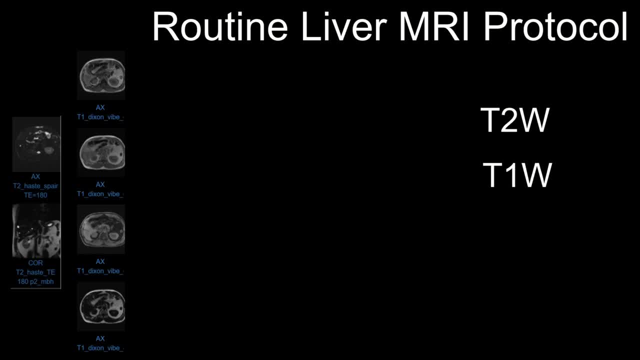 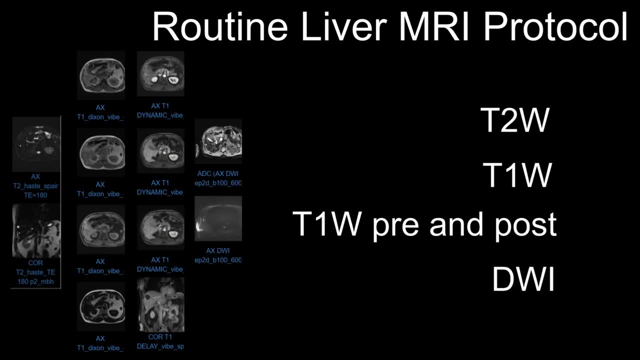 out of phase with calculated fat only and water only images. We have our pre and post gadolinium T1 weighted images, done with fat suppression, and then we have our diffusion weighted images. Okay, so before going through my approach, I want to briefly introduce gadolinium based contrast. 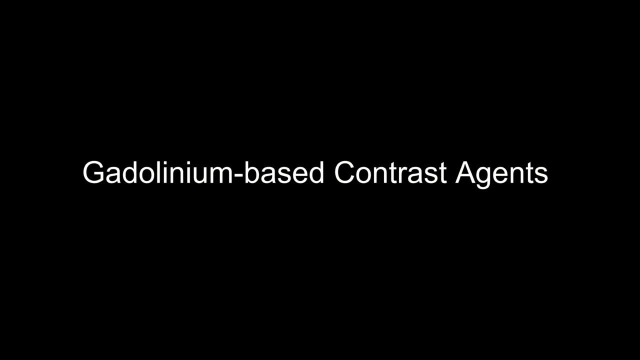 agents that we use in liver MRI. so as a practical starting point, you should know the following. so in MRI in general, we most commonly use extracellular contrast agents, and when most people colloquially refer to gadolinium or gad, they really mean one of these extracellular 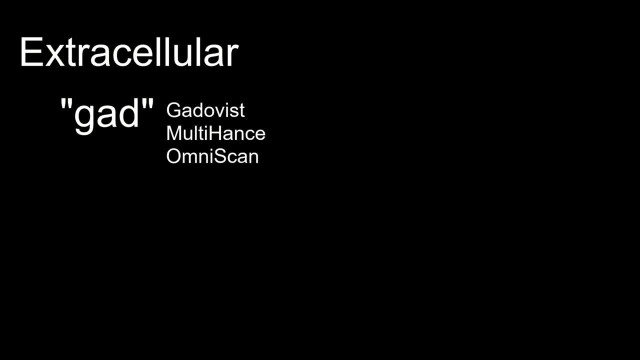 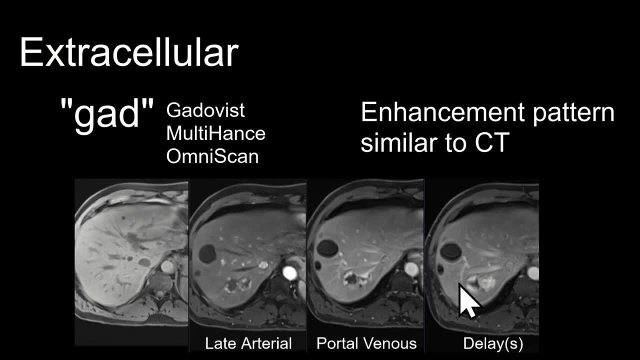 contrast agents like gadavist. so these are excreted by the kidneys and on imaging they behave very, very similarly to iodine-based contrast agents in CT. so in general you can apply what you know about IV contrast enhancement patterns from CT to MRI with quote-unquote gad. 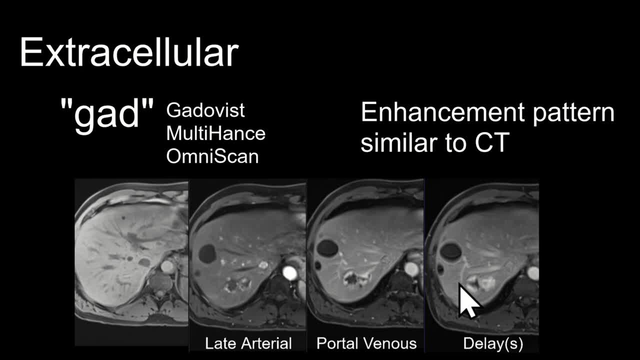 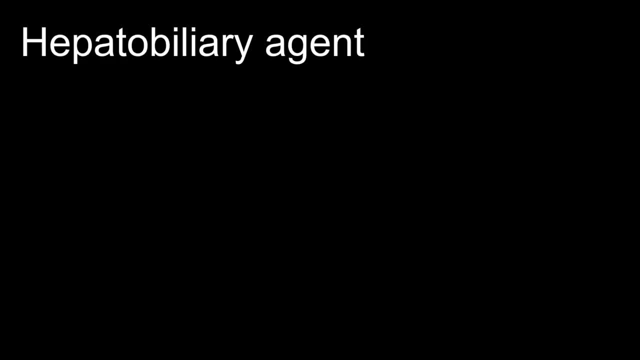 so for routine liver imaging we use these extracellular contrast agents, but there are some circumstances where it's helpful to use a hepatobiliary specific contrast agent called gadazetic acid, trade name eavist in the US and premavist elsewhere. I'll use premavist because 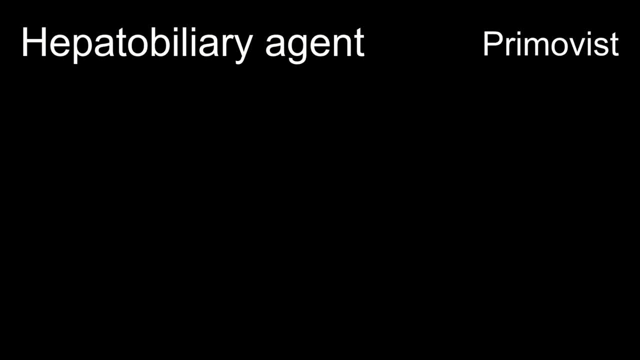 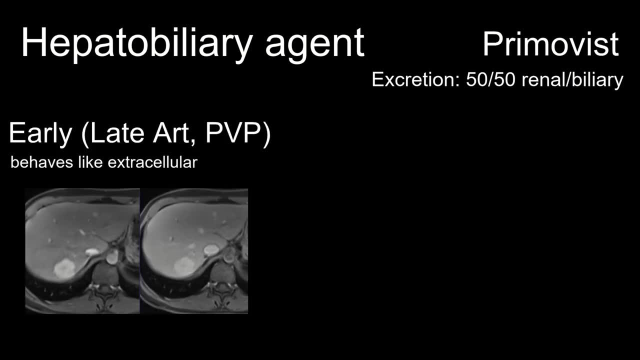 I'm from Toronto, Canada, so premavist is excreted both by the renal and hepatobiliary system about 50- 50 and so early after injection it behaves like an extracellular contrast agent that you're used to, but over time the liver cells will take up premavist, mostly due to a transporter called OATP1B3, and then begin to 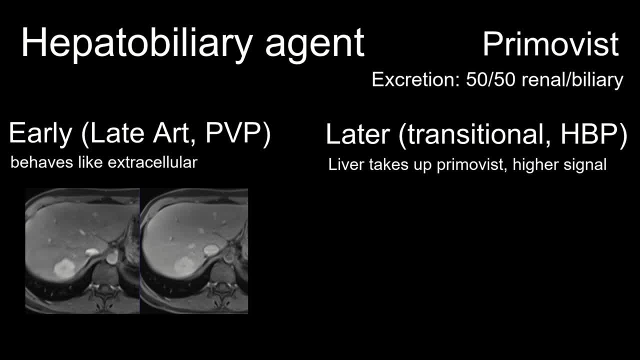 excrete it in the biliary system. so over time the background liver gets brighter, so the appearance may be different than with extracellular contrast agents. if we wait 15 to 20 minutes, an image. the liver will be very bright and the biliary system will be even brighter, since it's filled. 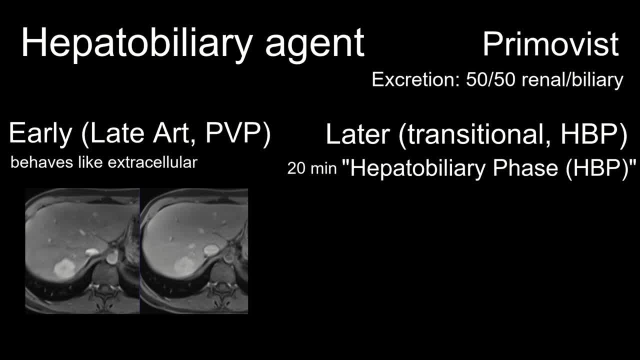 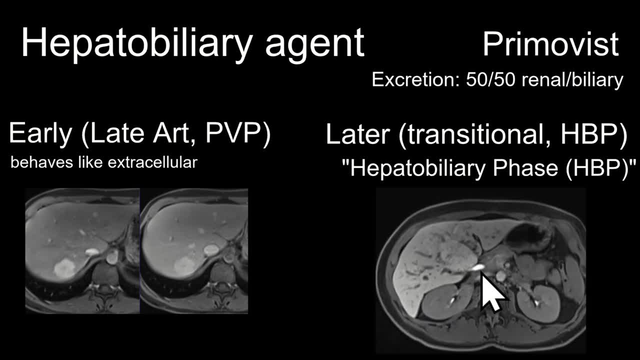 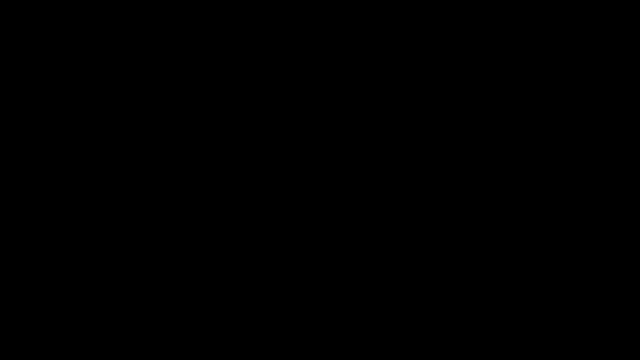 with excreted contrast. so this gives rise to the name, the so-called hepatobiliary phase. so notice that the biliary system here on this hepatobiliary phase sequence is very, very bright. in the background liver is also very, very bright. so there are many clinical scenarios where this can be useful and beneficial clinically, and so 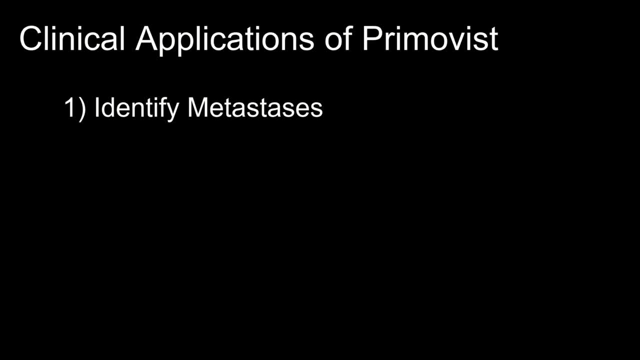 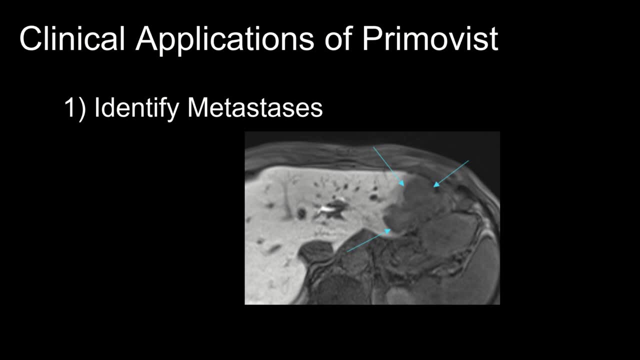 to name a few common uses, one to identify metastases. so if the background liver is very bright on hepatobiliary phase because of the primavis uptake, focal metastases and other non-hepatocyte containing lesions are going to be dark. so this is important in certain types of. 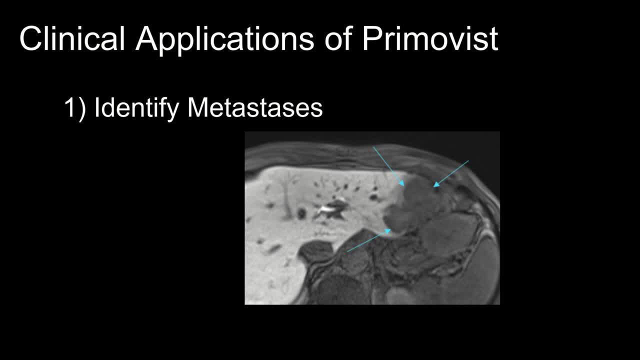 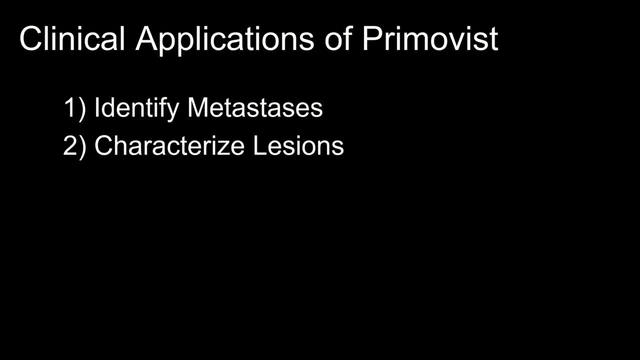 cancers like colorectal cancer, where hepatic metastases can be cut out with curative intent. so we need to identify all of the metastases. secondly, primavis can help with the characterization of some lesions. so lesions that express OATP1B3 will also take up primavis, the classic example. 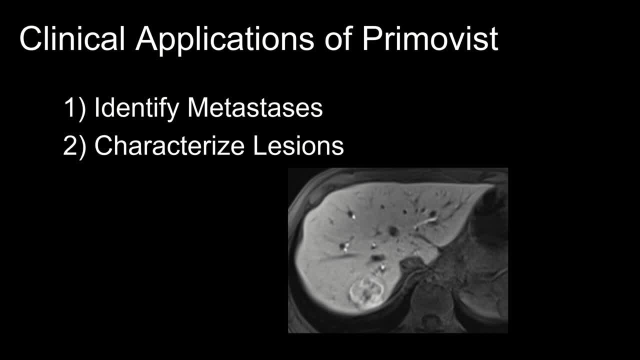 to know for now is FNH or focal nodular hyperplasia, which will be iso-intense or hyper-intense to background liver on hepatobiliary phase. but there are others that we'll touch on in the course. and then three to look at the biliary system. the biliary system is a system that is used to 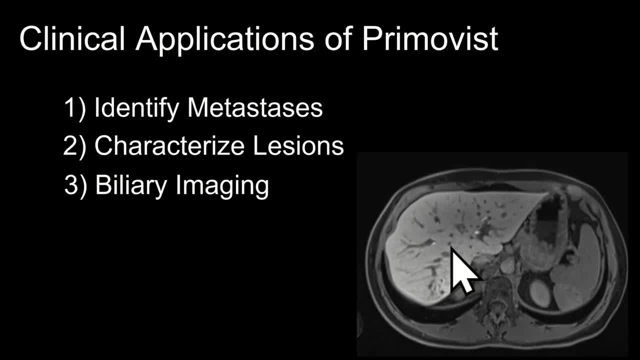 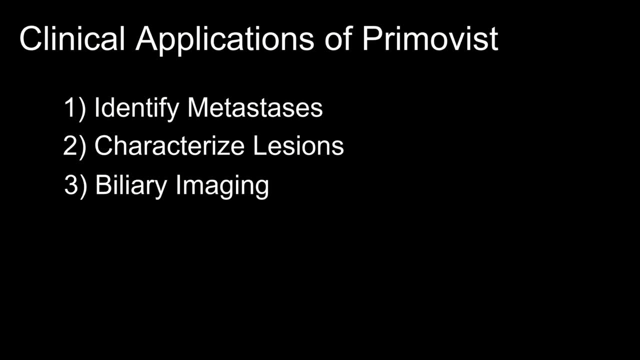 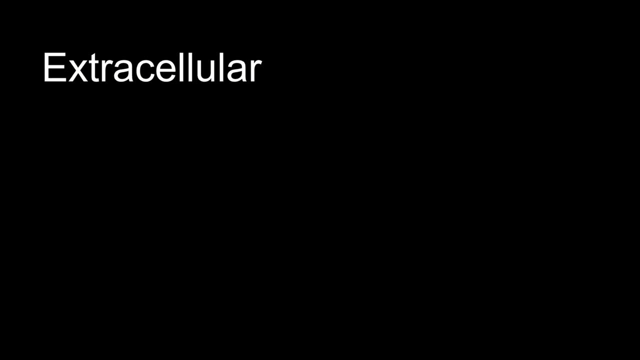 define the biliary anatomy and assess the biliary system, including for bile leaks, for example. so if that's all too much for now, just remember that extracellular agents, which are used in the vast majority of cases, behave like iodine-based CT contrast agents, so we can apply the enhancement. 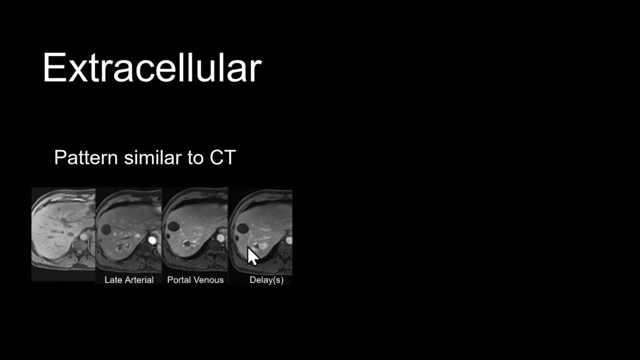 patterns. we know from CT to MRI with these agents also. we have the hepatobiliary system that is used in the vast majority of cases. we know from CT to MRI with these agents also. we have the specific agents, like primavis, that have certain clinical indications that behave similar to 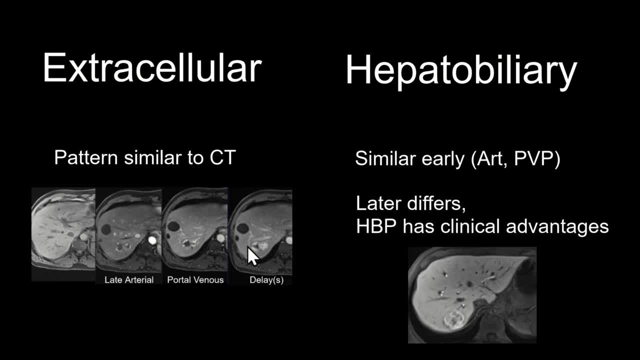 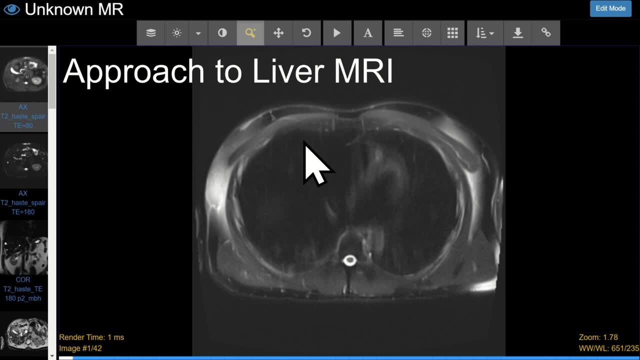 extracellular contrast agents early on, but over time the enhancement patterns can differ from what we expect to see with quote-unquote GAD. so now that we've covered the basics, I'm going to briefly take you through my practical approach to interpreting a liver MRI. then we'll cover the 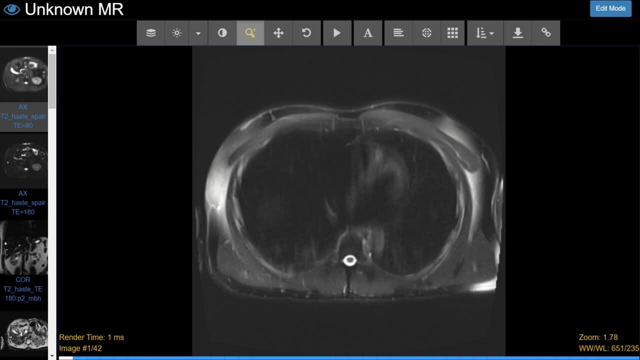 case of the 20 year old male patient from the start of the video together. so again, there are a lot of sequences and everyone has their own way of looking at the liver, so I'm going to go through my practical approach for the real world. so step one is to know the history of the 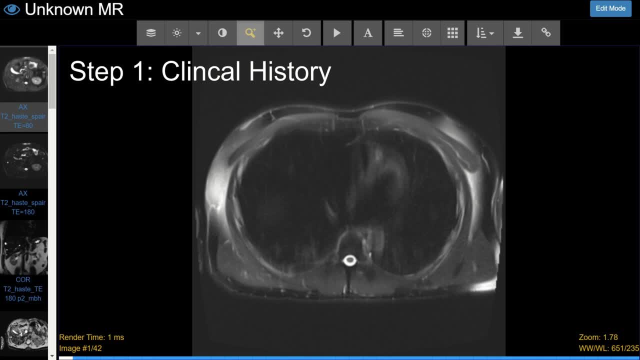 patient. so before looking at the images, it's important to know the clinical history, because the history completely changes how we interpret the images. most importantly, one I want to know: is there a history of known malignancy, which will increase the chance, of course, that there are liver metastases? the type of malignancy is also important. for example, we may expect: 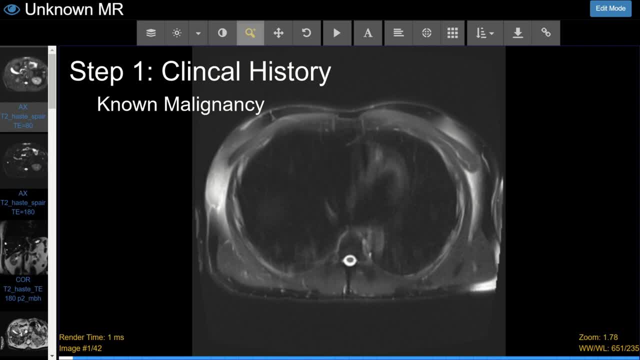 hypervascular metastases and things like RCC, neuroendocrine tumors, melanoma etc. and hypovascular metastases with most others, including colorectal two. I want to know if the patient is at high risk for HCC, most importantly a history of cirrhosis, chronic hepatitis B or prior HCC. if yes, to any of 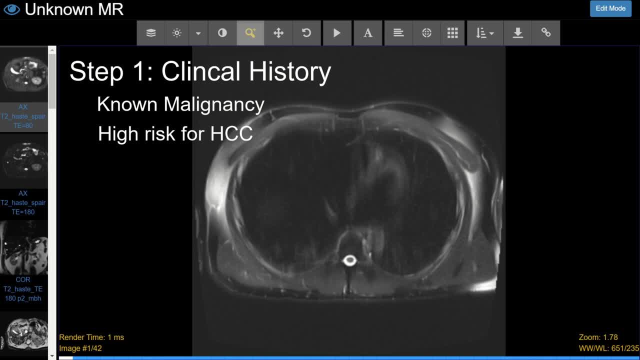 these. we're going to interpret focal lesions in the liver completely differently because the chance of HCC is significantly higher than in someone who does not have these risk factors, and we'll discuss that in detail in the course itself. and then three: any other relevant history, ie prior. 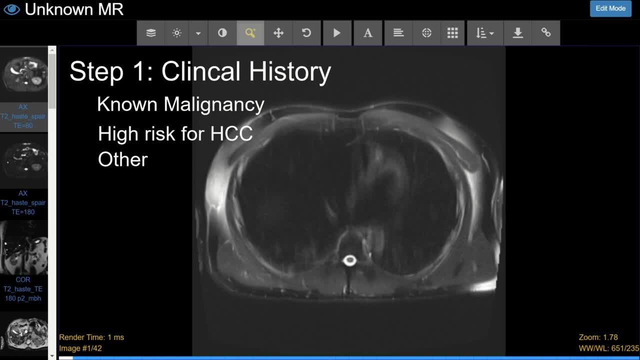 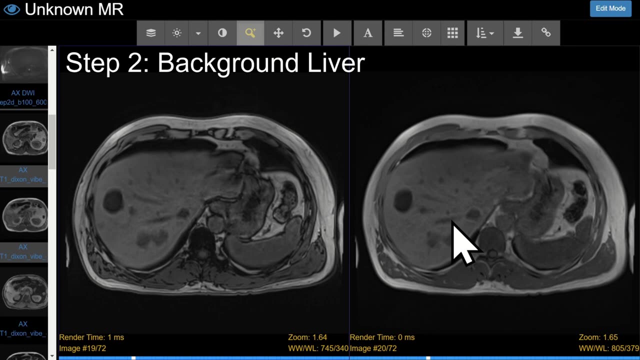 medications like chemotherapy, oral contraceptives, etc. and other relevant systemic disorders, and we'll touch on some of these important things in the relevant cases in the course. okay, and so step two is to start looking at the images, starting with the background liver, and I start looking at the background liver since, again, the presence of liver disease may change how. 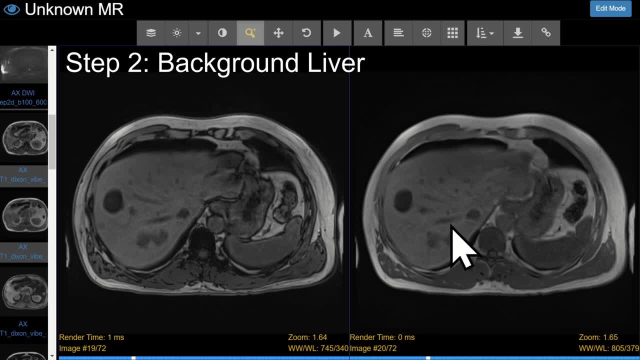 we interpret focal lesions in the liver. so, for example, if we see frank soros's, then we know that the risk of HCC, for example, is higher. so when I'm looking at the background liver, I start by looking at the internet of phase images and I'm looking for signal abnormality on the internet of phase. 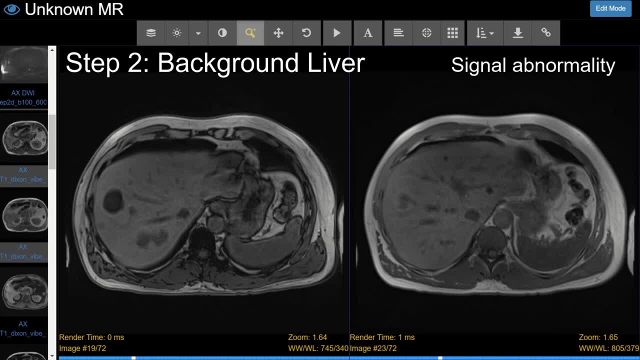 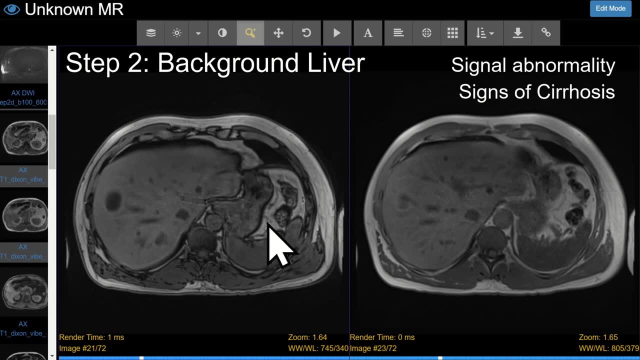 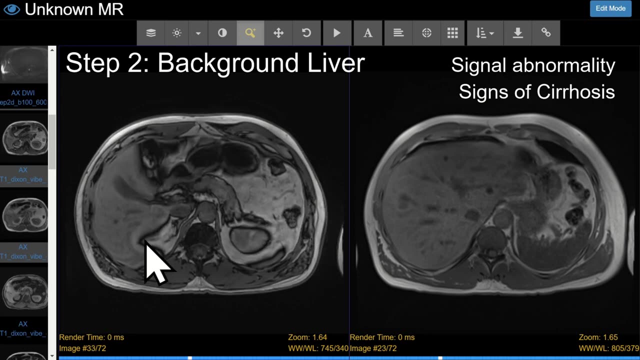 images. so specifically for fat content and iron, ie for hepatic steatosis or iron loading in the liver, the liver. I'm also looking at the morphology of the liver on these images, including the liver contour, specifically on the out-of-phase. So notice that the contour is nicely outlined by 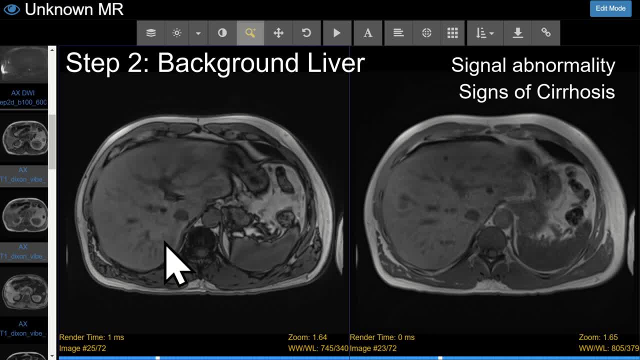 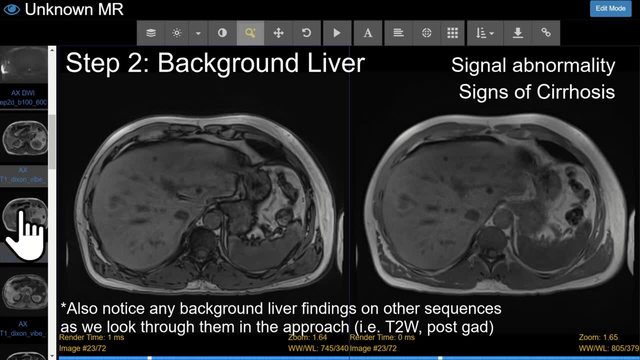 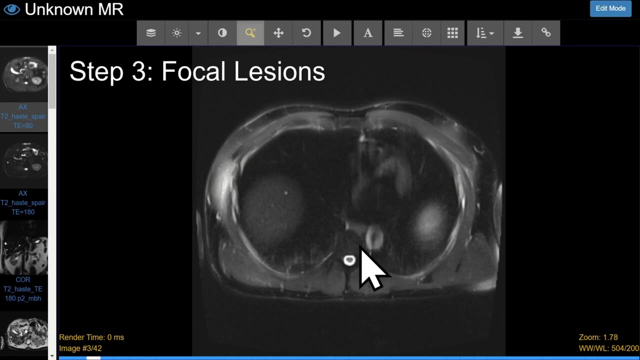 the Indian ink artifact and I'm looking for signs of cirrhosis like lobar redistribution and frank surface nodularity. So for this case there's no background signal. abnormality in the liver. Next I start looking for focal lesions. So I start by looking at the axial fat set T2. 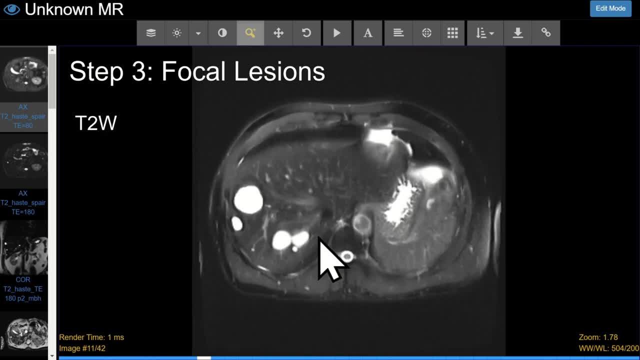 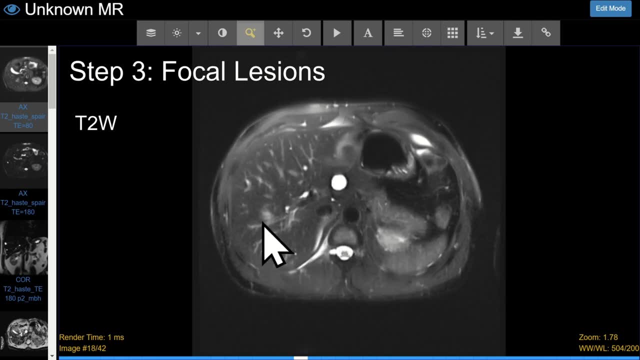 weighted images. Again, you'll notice that the normal background liver is pretty dark on the T2 weighted images and most but not all liver lesions are going to be relatively bright compared to the background liver. I should say that any time in this approach if I see something abnormal. 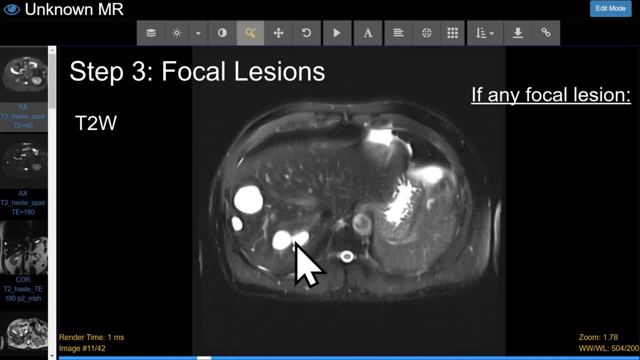 or anything focal. I then look at that lesion on all of the sequences to characterize it first. I then look at that lesion on all of the sequences to characterize it first. Specifically for things I want to know: what does it look like on pre-contrast images? 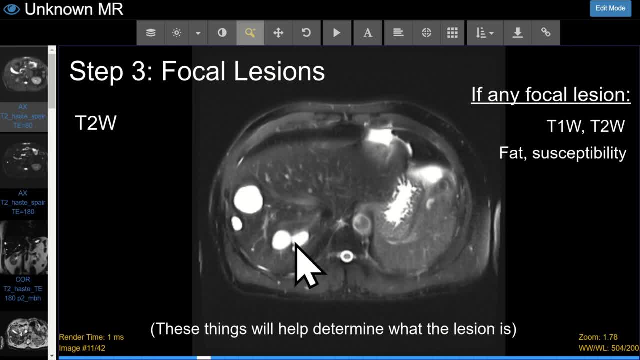 aka T1 and T2 weighted images. Does it contain fat, Does it restrict diffusion And what is the enhancement pattern over time? So for now I'm going to take you through a general approach, but remember, any time you see anything focal on any sequence you want to characterize and 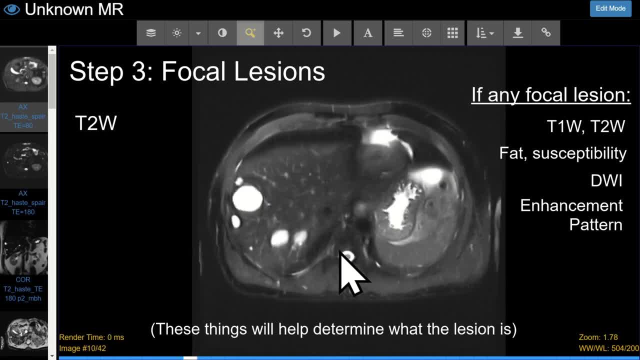 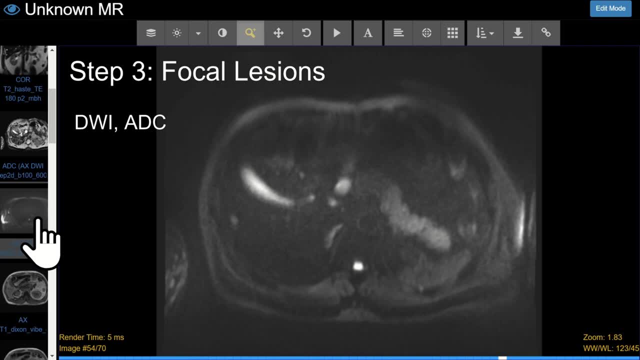 know those four things. So once I've looked at the T2 weighted images, a lot of people will go to the T1 and pre- and post-contrast images. but next I'm going to look at the T2 weighted images. Next I generally jump directly to the diffusion weighted images and I have a quick look through. 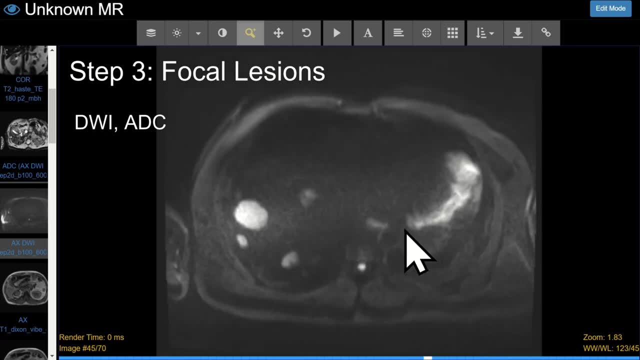 for any obvious lesions on both the low and high B-value images, specifically looking for any lesions that are restricting diffusion. So diffusion is a great sequence. Certain types of metastases are going to stand out best on the diffusion weighted images and may be a lot more difficult. 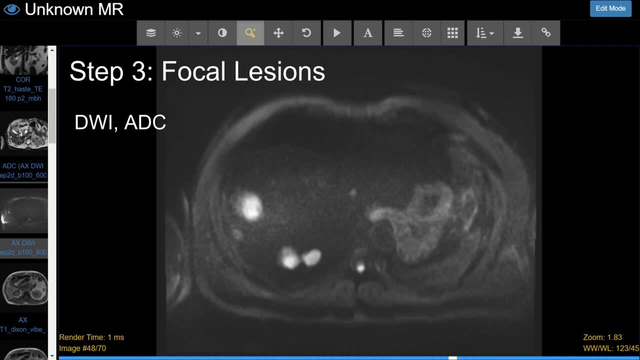 to see on other sequences. With that being said, there are other malignant lesions that may not be very well seen on diffusion weighted images, But I like it a lot because it gives you a quick overview And the rule of thumb for DWI in the 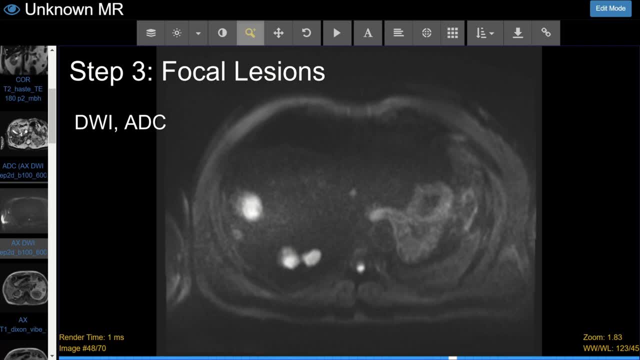 liver is. if you see something and it restricts diffusion, that's very helpful. But if you don't see anything on DWI, that doesn't necessarily rule anything out. Again, if you see a focal lesion on these sequences, you want to look at its characteristics on all sequences: the T1 and 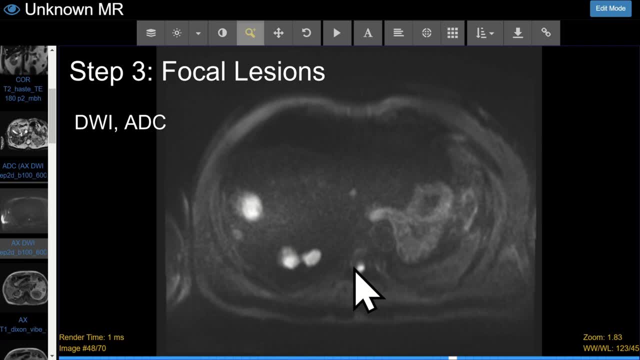 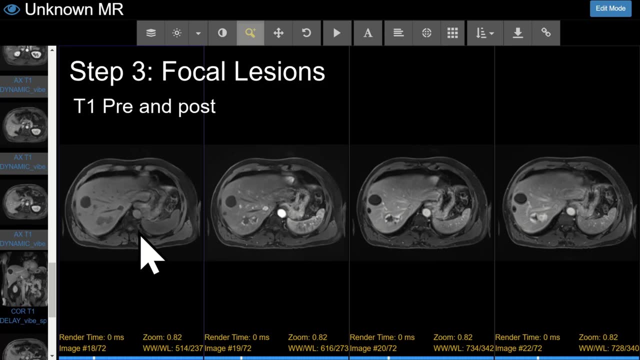 T2 weighted signal. Does it contain fat, Does it restrict diffusion And what is the enhancement pattern over time? Lastly, I look at the T1 pre- and post-contrast images And the approach to this is somewhat similar to multiphasic CT. On the pre-contrast, fat-saturated or fat-suppressed. 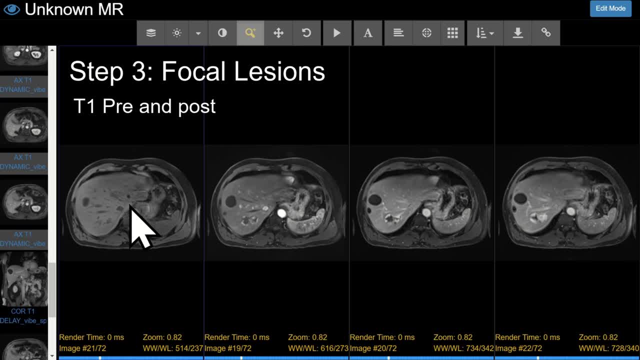 images. I want to look for focal lesions, including for lesions with intrinsic T1 hyperintensity, which may indicate hemorrhage, proteinaceous material or melanin. Again, you always want to make sure that the arterial phase is well-timed And then look closely for the T1 hyperintensity. 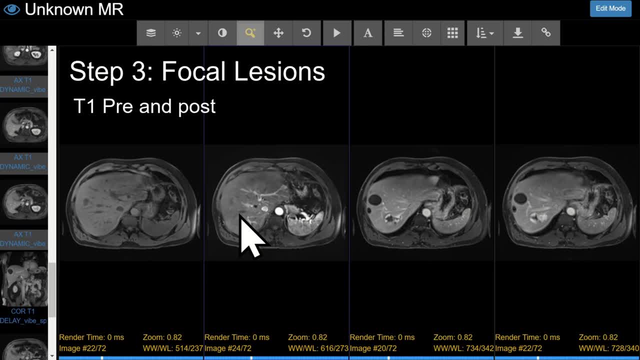 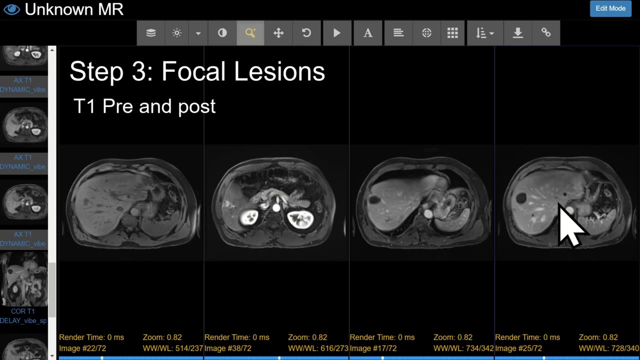 or hypervascular lesion lesions on late arterial phase. This is something that you're going to take your time with, especially if the patient is at high risk for HCC. On portal venous and delayed phases, we're going to be looking for relatively hypovascular lesions And then once again of. 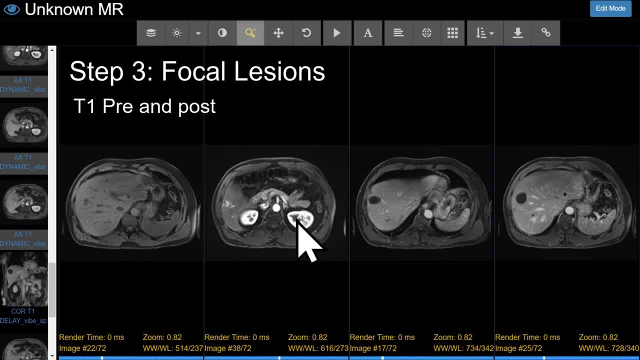 course, if you see any focal lesion anywhere, you want to characterize it again by looking at the T1 and T2 weighted signal pre-contrast, whether it contains fat or susceptibility, whether it restricts diffusion, and then the enhancement pattern over time. And, of course, 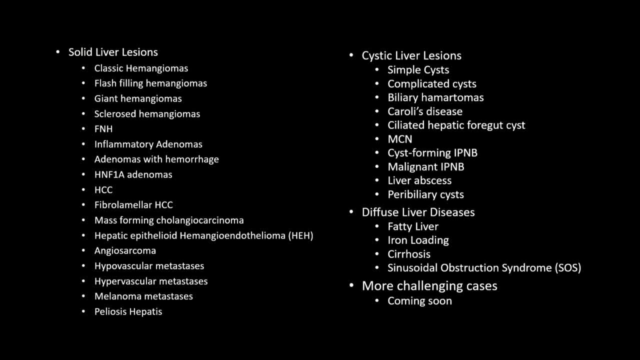 in the liver MRI course, we're going to cover in detail the typical appearance of all of the liver lesions that you need to know, And so then, if you know those characteristics, when you see a liver lesion on MRI in real life, you'll be able to note the four characteristics that we spoke about. 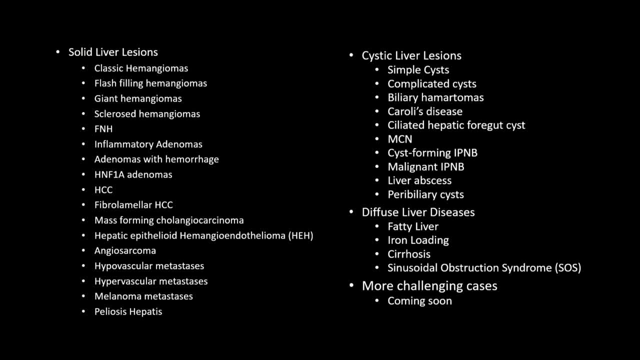 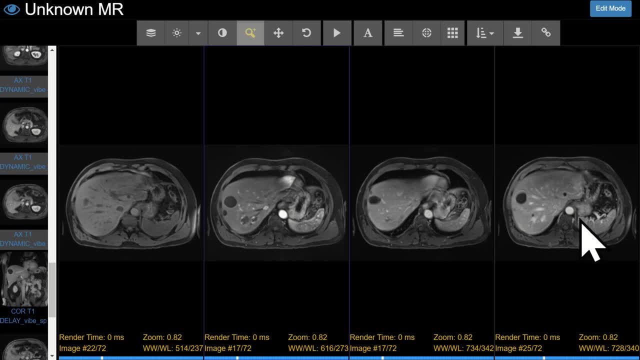 and then put the lesion into a box to know what that liver lesion is or if there's a differential between a couple of different types. Of course, after looking at the liver, we're going to look at the structures in the rest of the abdomen, which is all covered in the body MRI intro video with the link to that approach. 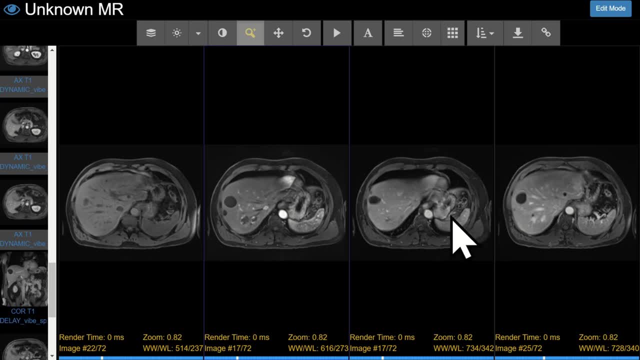 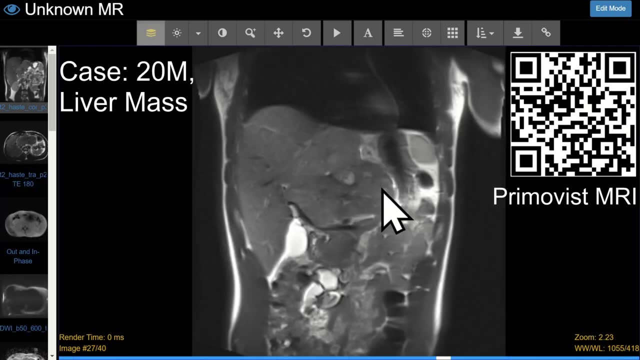 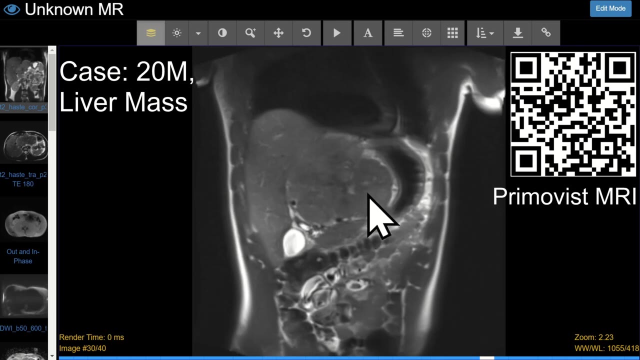 on the screen, And so we'll cover the biliary system, pancreas, other solid organs, etc. in more detail in future videos. Okay, so let's get back to this case that we introduced at the beginning of the lecture. So this is a 20-year-old male patient who presented with some abdominal 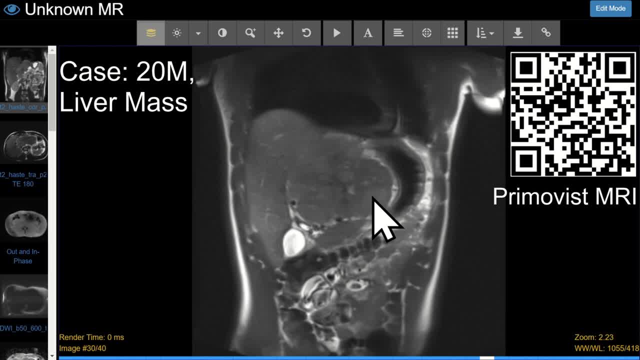 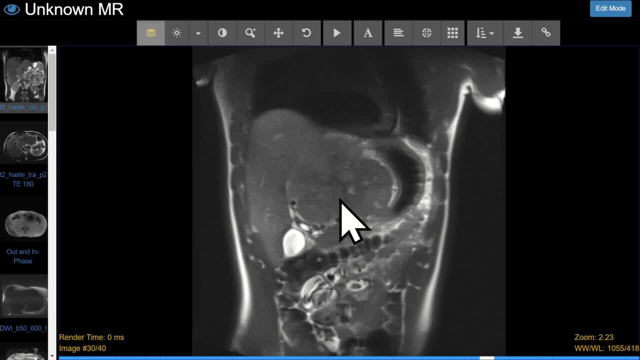 pain and there was a lot of pain in the abdomen And so we're going to look at the structure and was an- incidentally- discovered mass on ultrasound. that's being characterized on MRI. So there's no known history of cirrhosis and no known history of other malignancy And on the MRI images we 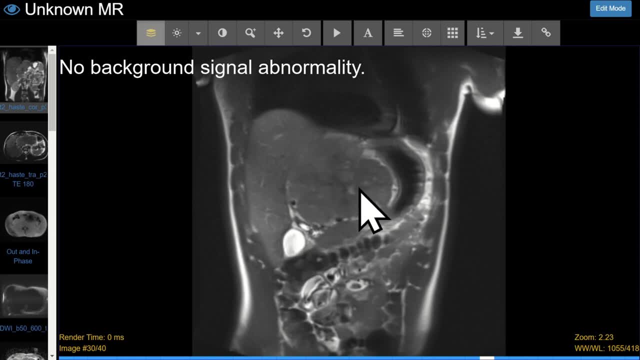 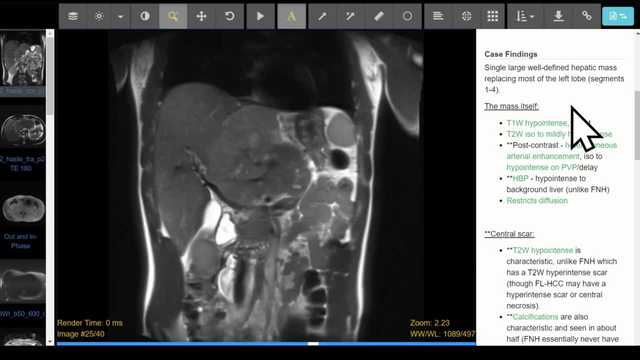 note that there's no background liver disease either. So let's go ahead and characterize the mass and look at what it looks like on all of these sequences and try to figure out what it is. So we'll jump straight to the answers from this particular case. So the mass itself. 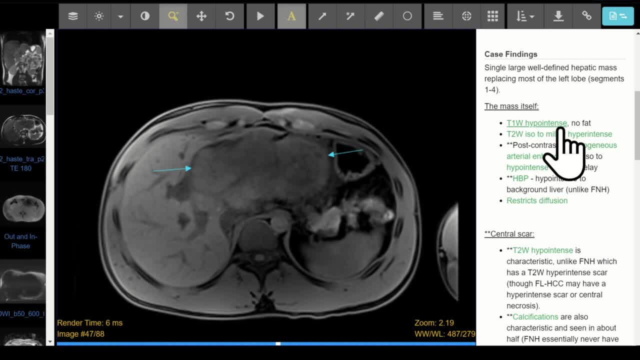 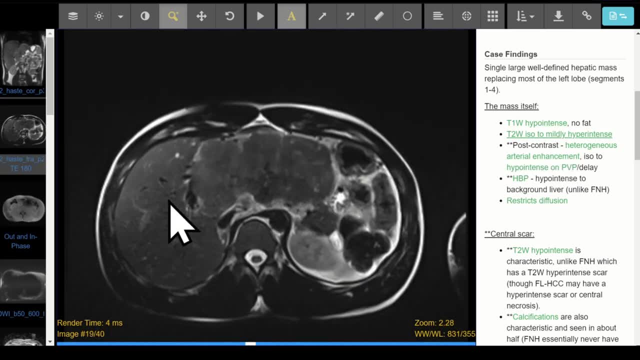 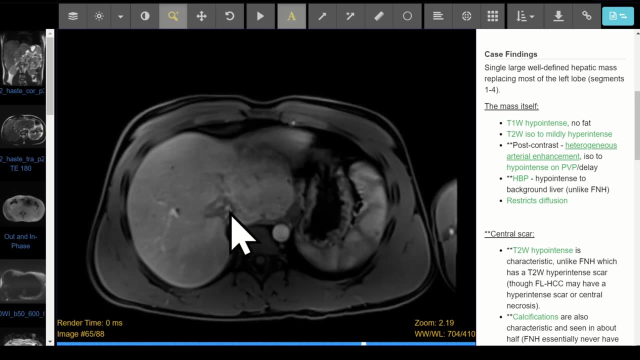 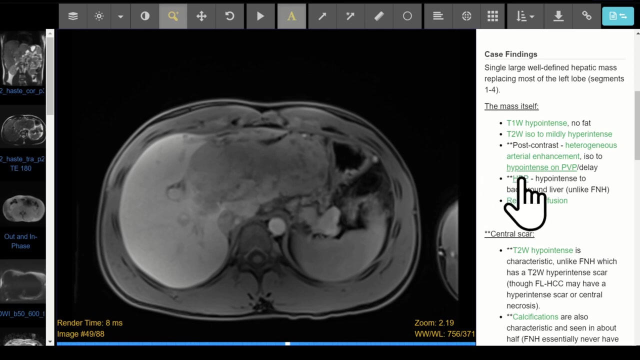 was T1 hypo intense and contained no fat. On the internet phase images it was T2, slightly hyper intense to background liver Post gadolinium. it demonstrated some heterogeneous arterial hyper enhancement and was relatively hypo intense on portal venous phase. This was a primavist study, And so the 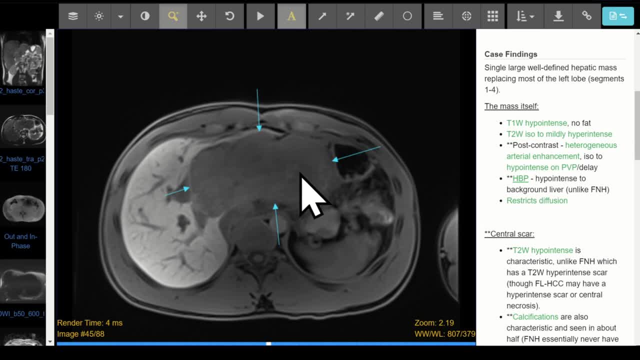 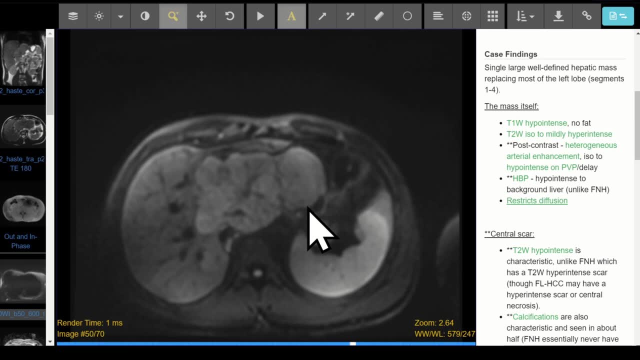 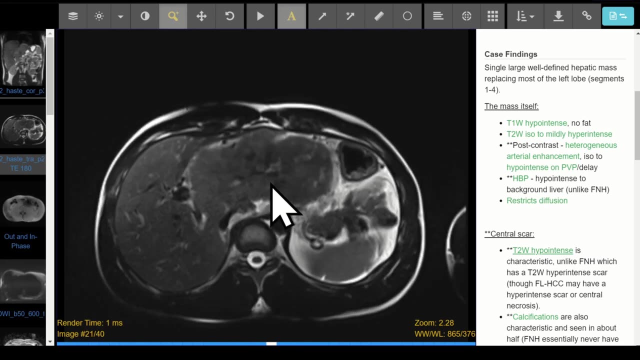 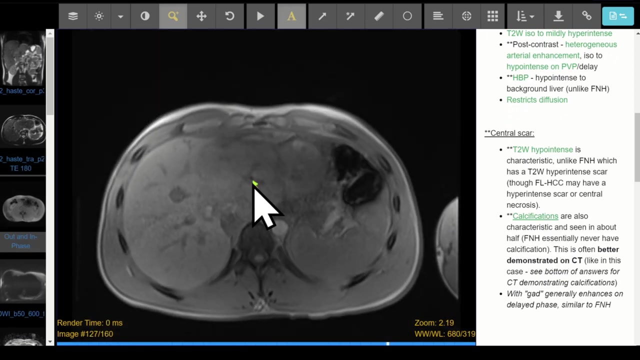 epitobiliary phase performed at 20 minutes, demonstrated that it was very hypo intense to background liver And so it was very restricted diffusion. Notice that the mass has a central scar within it That was very T2 hypo intense And also there were, or was, notes on the internet of phase images of this little focus of 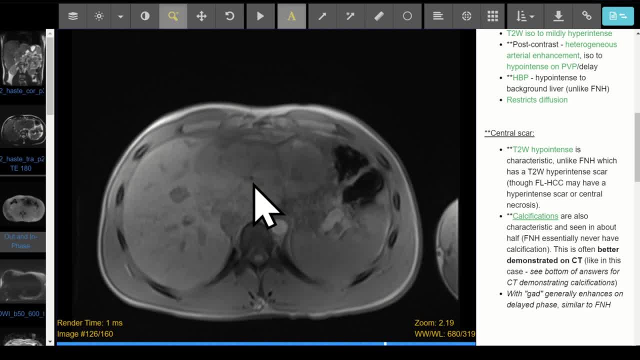 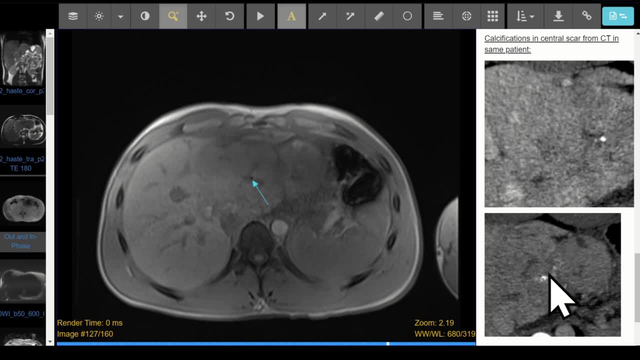 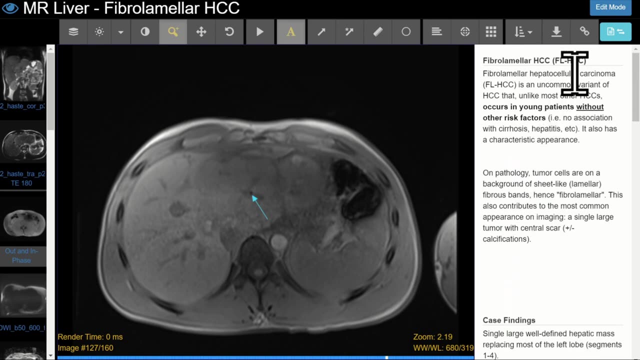 susceptibility artifact that was corresponding to calcifications that were better seen on the CT. So if I scroll down here you'll see the calcifications better seen on CT within the scar. So this was biopsied and came back as malignant, namely a fibrolamellar HCC. 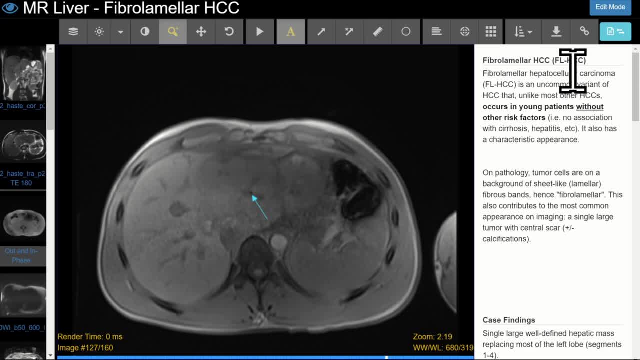 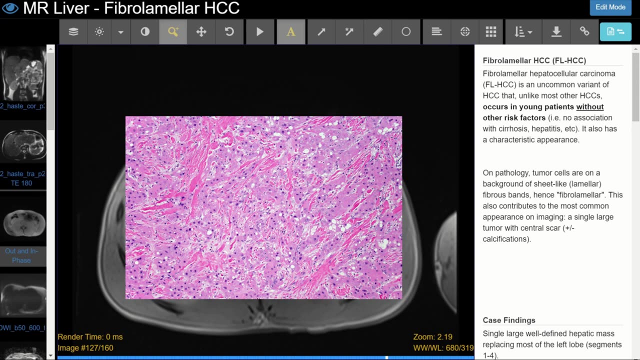 which is an uncommon variant of HCC that, unlike most other HCCs, occurs in young patients without other risk factors for HCC. So, on pathology, in fibrolamellar HCC, the tumor cells are on a background of sheet-like or lamellar fibrous bands, So hence the fibrolamellar And the 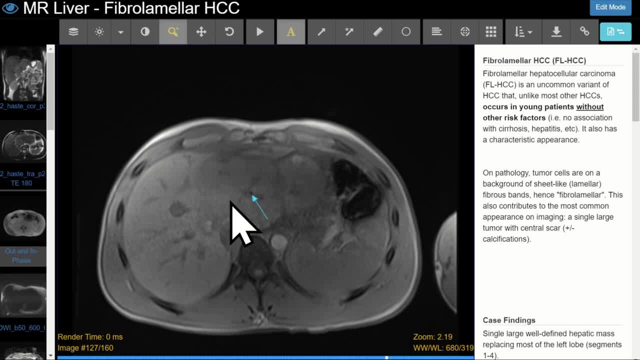 imaging appearance in this case is typical of fibrolamellar HCC. So here we have a single large tumor with a central scar, and the central scar can make it difficult to differentiate from FNH, which is benign. Of course. calling this mass and FNH would be detrimental to the patient. 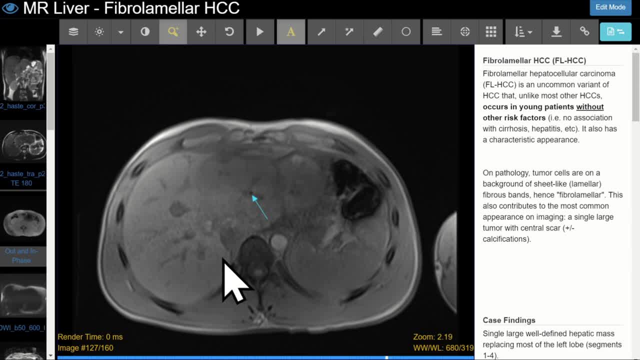 But of course there are a few key features that are going to help you differentiate FNH from fibrolamellar HCC that are covered in detail in the course. The most important and classic that we showed here are the fibrolamellar HCC and the fibrolamellar HCC. So here we have a single large 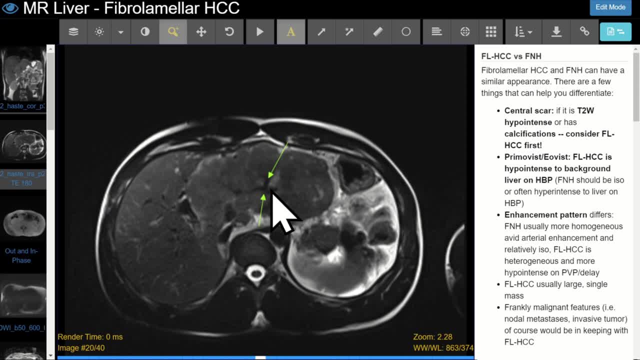 tumor with a central scar And the central scar can make it difficult to differentiate from FNH, which is the central scar being T2 hypo-intense in fibrolamellar HCC. In FNH it tends to be T2 hyper-intense, The calcifications that we showed you on the CT within the mass. So calcifications. 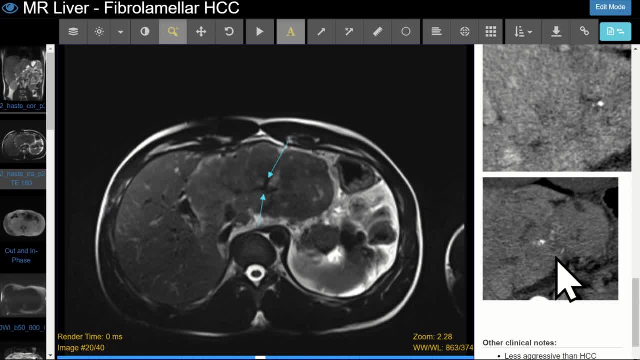 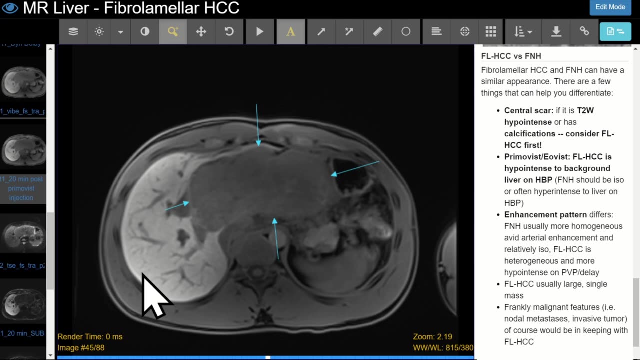 are common in fibrolamellar HCC but almost never seen in FNH. And the calcifications again are what caused the susceptibility artifact that we saw on the MRI in-phase images And the mass was very hypo-intense to background liver on hepatobiliary phase. So of course FNH is. 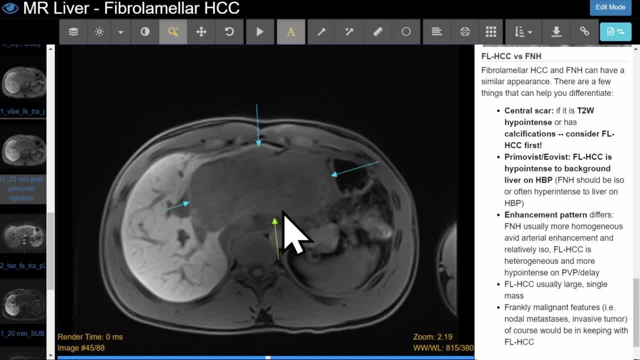 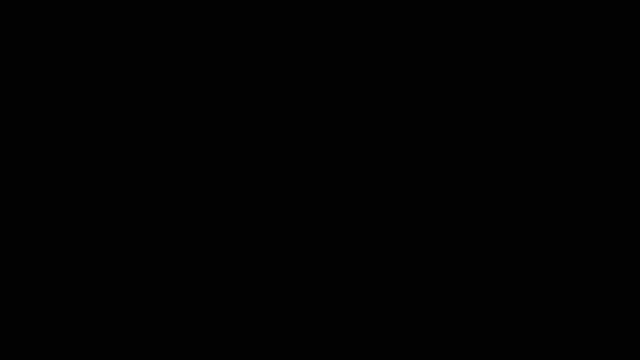 characteristically iso-to-hyper-intense to background liver on hepatobiliary phase. Of course, if there are other frankly malignant features like invasion of surrounding structures, metastatic nodes, etc. we would think malignancy as well. Next, I want you to apply what you've learned in this video by taking the liver MRI cases in our 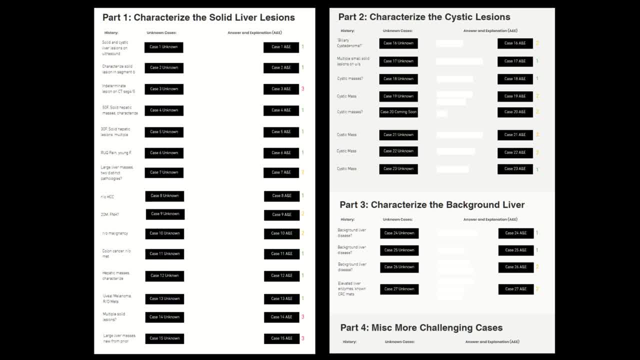 liver MRI course, Which includes all of the most important pathologies that you need to know, walkthroughs of imaging findings and everything that you need to know about each case. So we cover how to characterize focal, solid and cystic liver lesions, diffuse liver diseases and some more challenging cases, And to access the rest of the course. 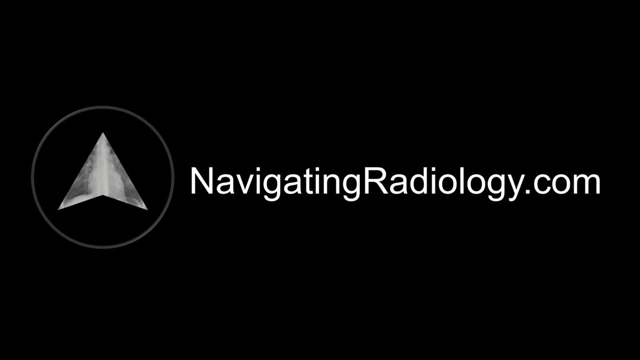 visit our website at navigatingradiologycom. Thanks for listening and I hope you enjoy the rest of the course. I'll see you in the next video. 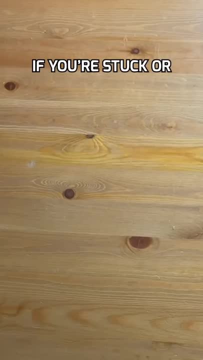 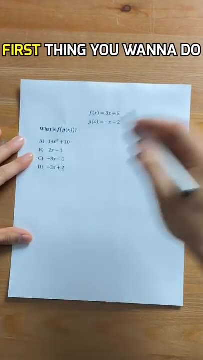 Here's how you can figure out the answer to any question on a test. If you're stuck or running out of time, use this guessing strategy, For example. let's look at this math question. First thing you want to do is eliminate the outlier, because chances are. 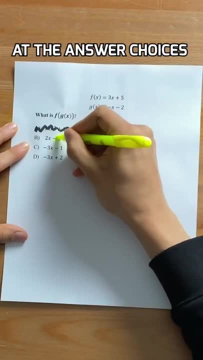 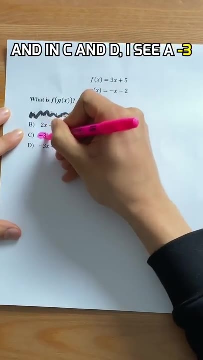 that's not even the right answer anyways. Then you want to look at the answer choices and find any similarities. So in B and C I see a negative 1, and in C and D I see a negative 3.. Chances are, the answer is most likely the one with the most similarities. so you want to pick C in this case. 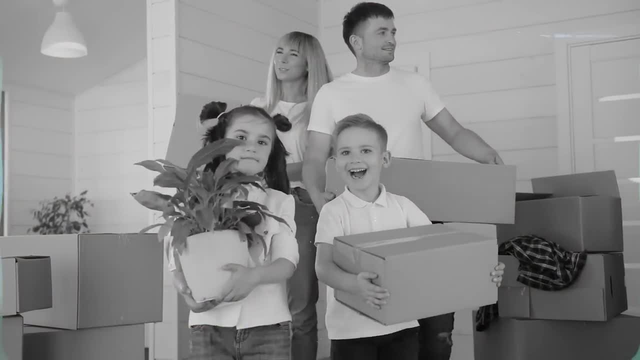 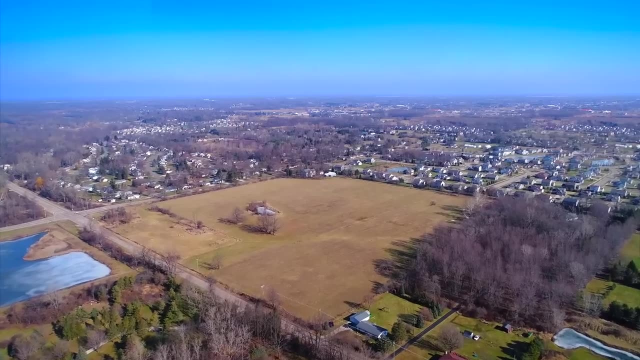 affordable to the average American, at least in most of the markets across the country. But there are still good deals to be had at reasonable prices, And I actually found five great markets where the median sales price is less than half the national average, So that means they are less than $200,000.. I used a few criteria to pick these markets. Here they are. First, median sale price, like I said, had to be under $200,000.. The second thing is that the sale price has to be up year over year. As you all probably know, we are in the midst of a housing.